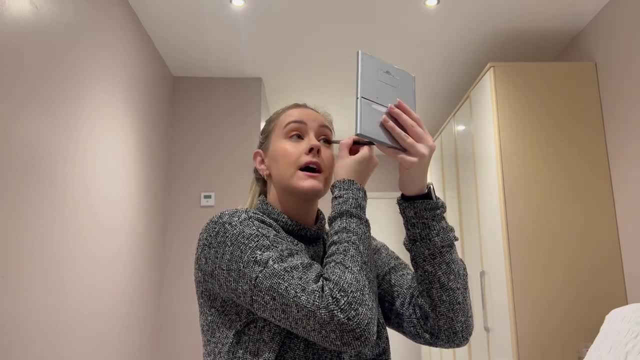 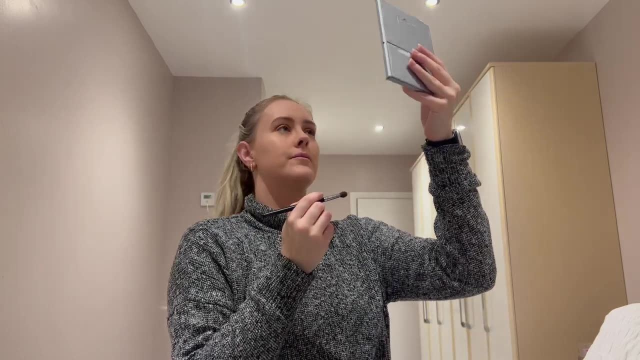 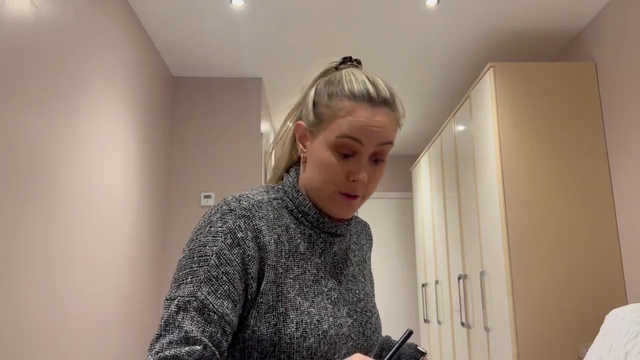 There's an airplane going by- Okay, the airplane is gone now- Yeah, so that has been quite challenging, let's say, because I've had to spend a lot of my time just doing data analysis. Sorry, I really can't see what my eyeshadow looks like and I don't want to go into work looking all crazy like a clown. 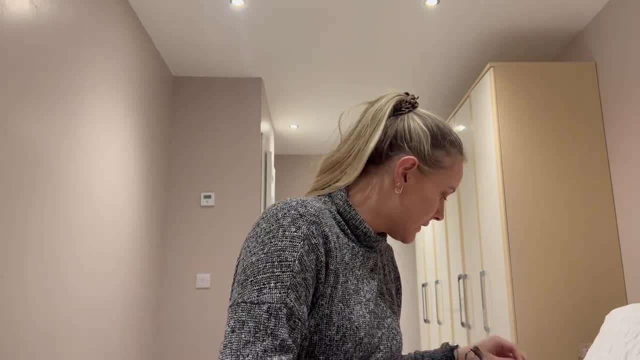 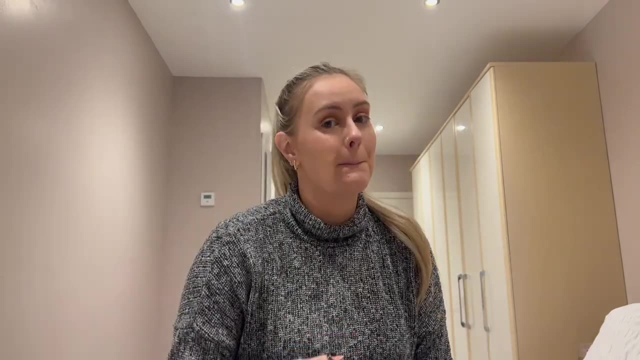 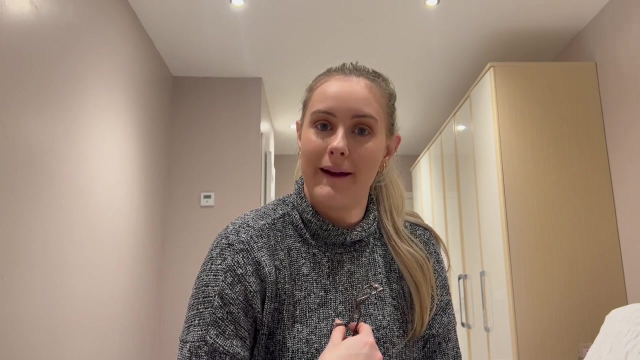 Yeah, so I have been focusing about 80% of my time on data analysis, which has been challenging because I've been staring at a screen, staring at numbers, staring at peaks, Staring at excel sheets and, yes, it is challenging for your mind. 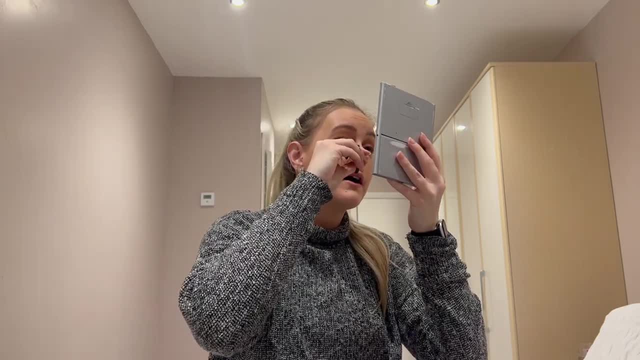 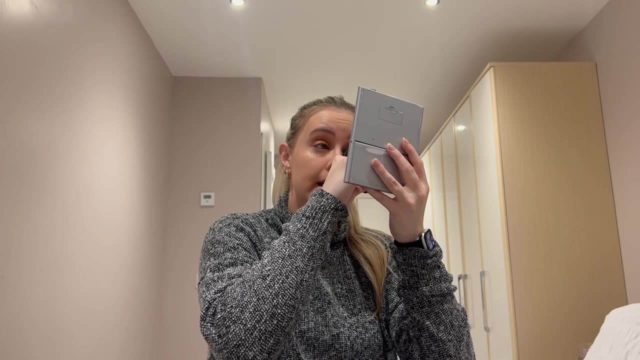 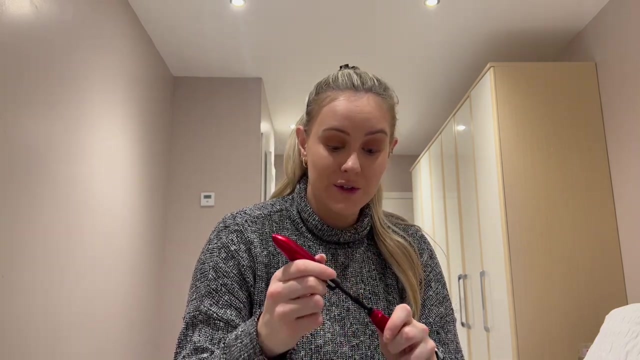 Alongside that, I've also been working on my method that I've told you about in a few vlogs. This is a method that I need to develop for when we get samples in, and I'm very pleased to say that the method has worked. finally, After trialling quite a few different methods, I have 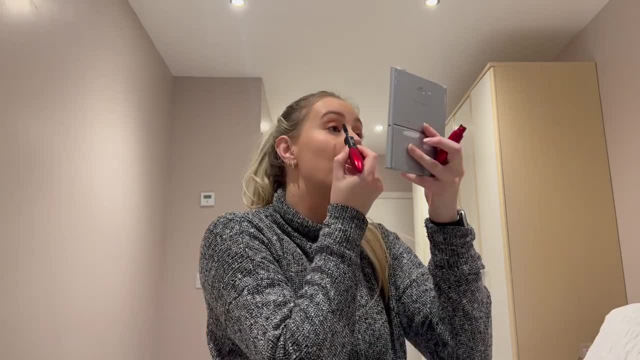 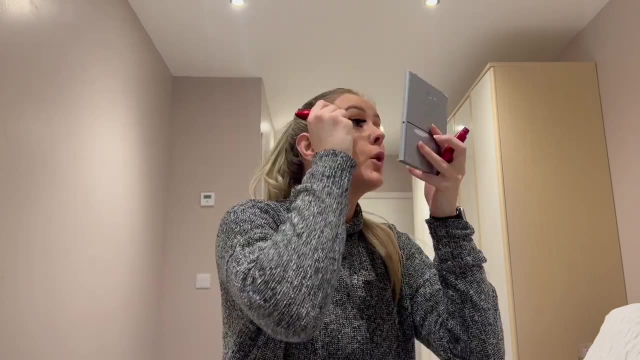 managed to get it to work, and I managed to get it to work very well, so I am very pleased about that. But yeah, I've been trying to juggle this data in amongst getting this method organised, which has been fun. Well, it's been very, very busy, to say the least. 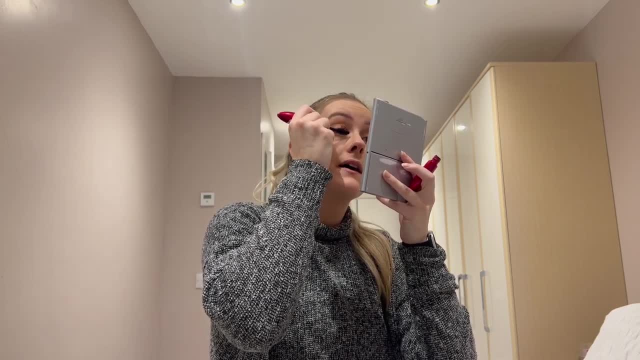 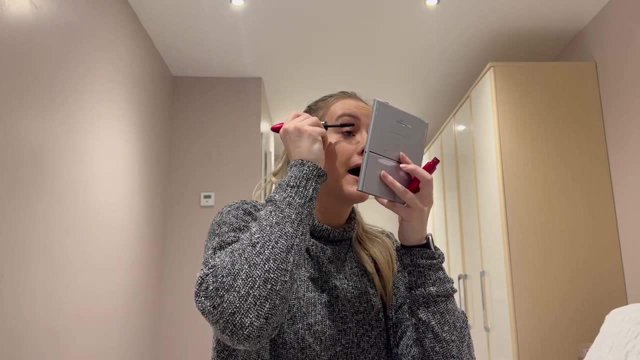 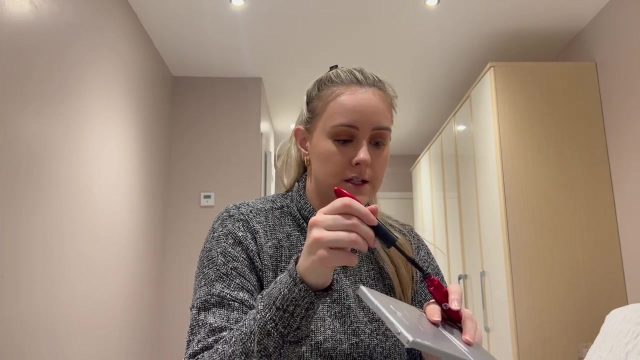 I was also a little bit stressed last week because I- well, it's actually Wednesday today and I took yesterday and Monday off because my boyfriend just came back from being offshore working for one whole month, so we wanted to take some time to spend together now that he's back. and I was quite honestly needing some time off because everything has been so hectic and busy at work. However, do you ever get that when you have days off planned and it happens to be that those days off are right in the middle of when you're at one of your busiest periods at work? 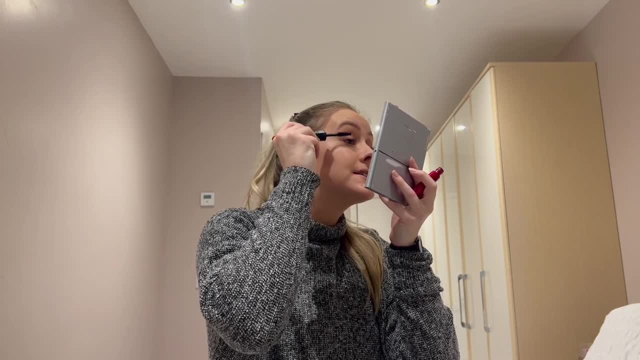 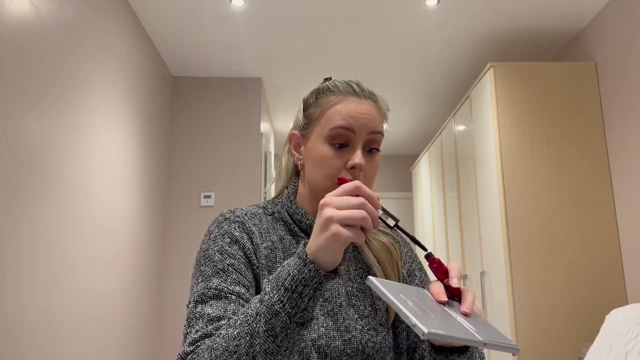 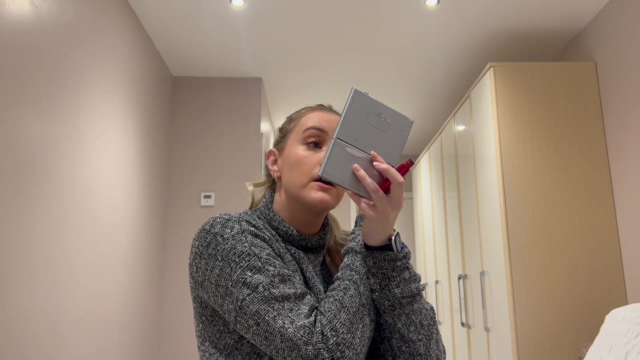 That is how it is felt because, yeah, I was quite stressed, thinking: oh, I have these days off, but I also have so much work to try and get done before this meeting and are these days off actually going to hold me back from reaching my goals of getting everything done before this meeting? So last week, I was a bit stressed, I have to say, and I did work quite a few hours over- well, over time, I guess, because I wanted to get myself in a good place by the end of Friday so that I could enjoy my weekend and enjoy my days off without thinking, you know, without being stressed over the weekend. 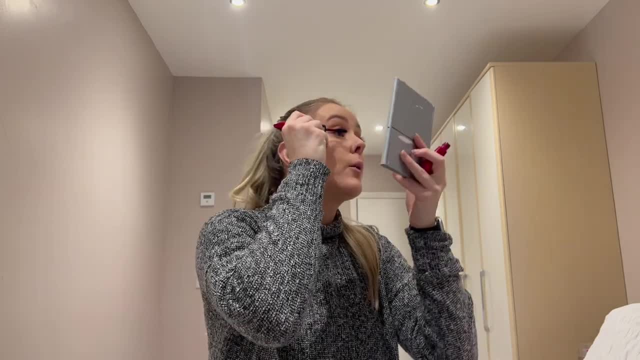 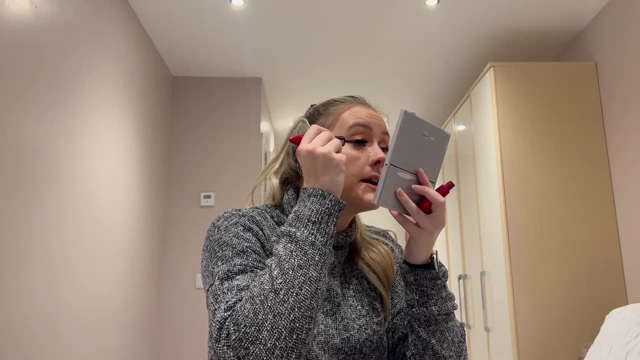 because I'm thinking, oh, I've got so much to do and I'm taking these days off. So I worked extra last week to try and put myself into a good position, and on Friday I was in a good position, I would say, and I have managed. 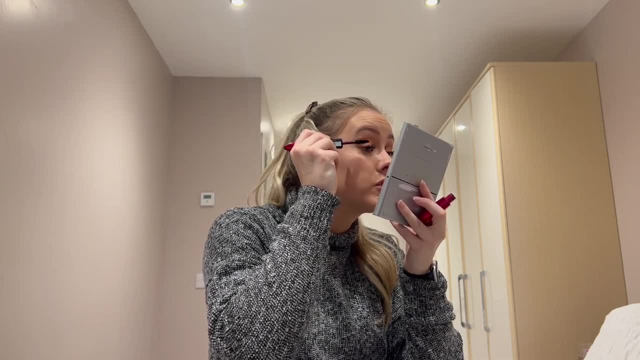 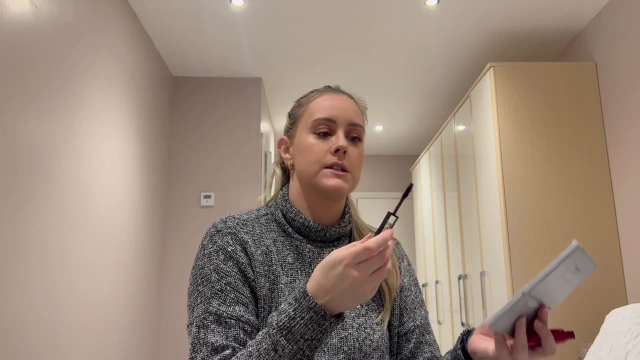 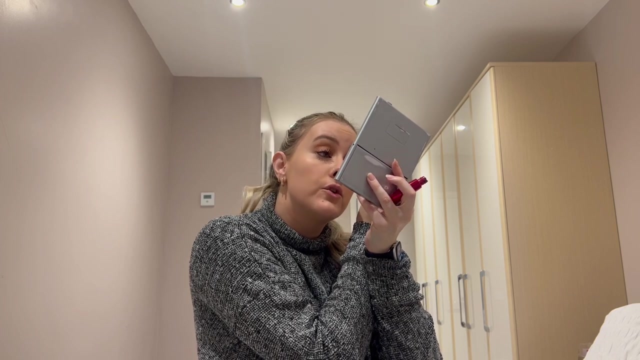 to enjoy my days off, but it is now time to return to work. This week, I'm probably going to be doing a mismatch of working from home and working in the lab. It depends if the samples that I was running while I was off if they worked out well, because this is the thing right When you look over your 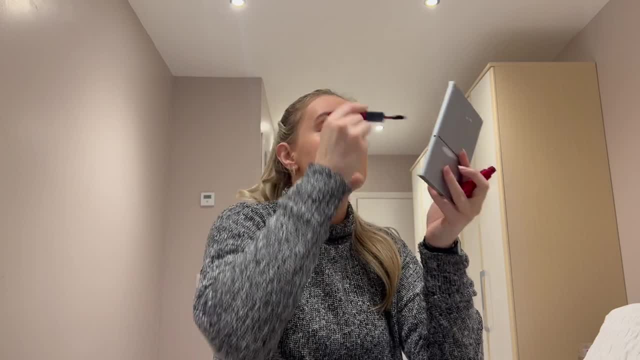 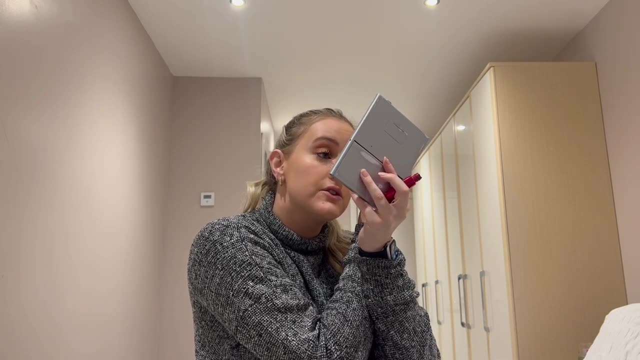 data. sometimes you don't know what's going on, and sometimes you don't know what's going on, You find that you actually need to rerun samples because something went wrong that you didn't realise at the time, until you've properly, like, dived deep into the data and you can see that 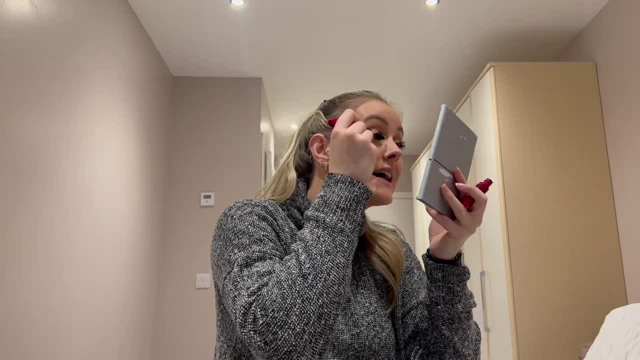 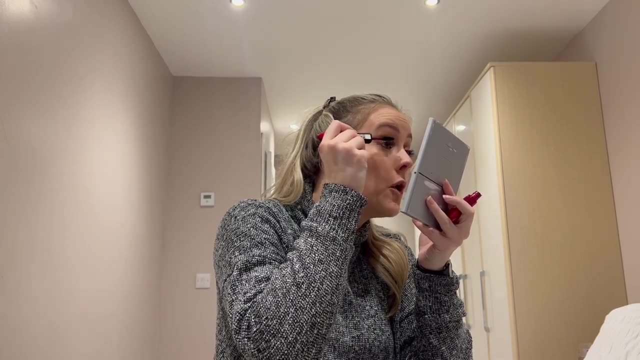 things aren't really matching up, so you need to redo stuff, and that is exactly what happened. So I was looking at data and realised that something strange happened that you wouldn't know, just from you know, glancing at the data briefly after you'd run the samples, 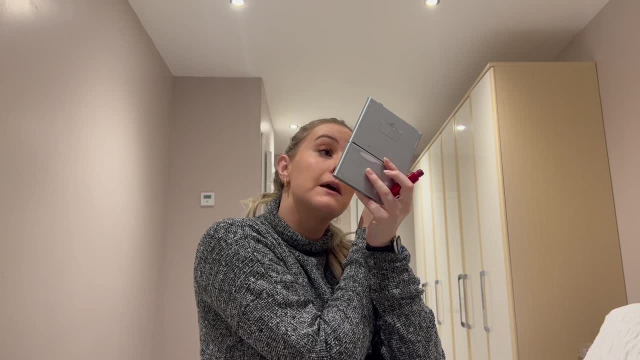 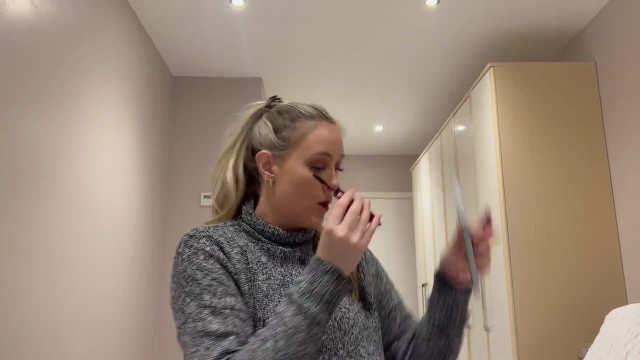 So I had to rerun quite a few samples, which means that I was waiting for that data in order to analyse and process it. So that data was running while I was off over the weekend and yesterday and Monday because my colleague Pat was going to be helping out with changing. 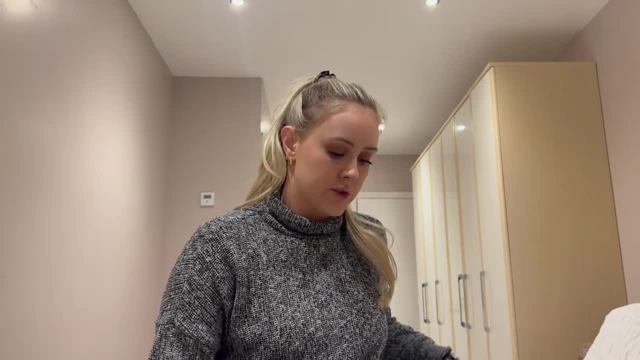 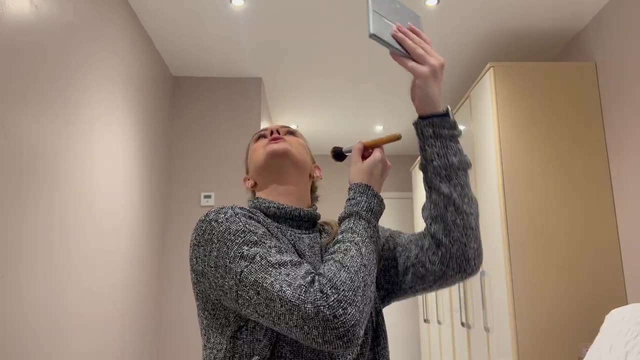 mobile phases on the LCFS and changing over samples and stuff like that. So that was very helpful. So all of my samples should be run now and they should be working- fingers crossed- and I should be able to analyse the last four sequences that were run and get them done by Friday and then 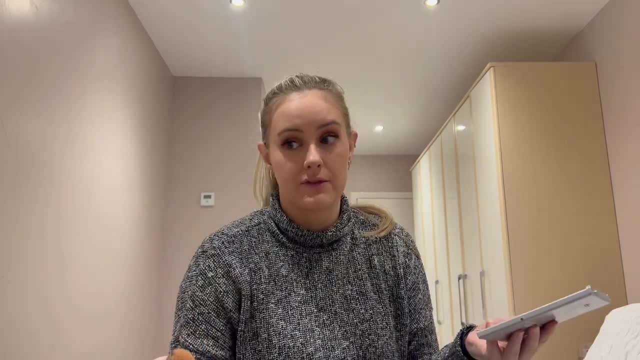 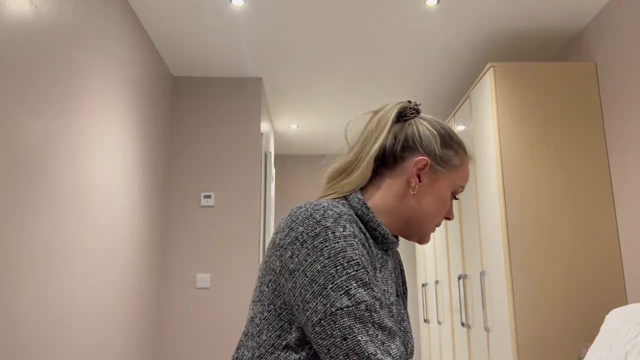 I'll be able to properly look at the trends of the data and try and make some graphs and see what has been happening in the river over the whole course of the year. So yeah, I'm going to take you along with me this week- well, this half week, since it's Wednesday- and just explain to you what I'm. 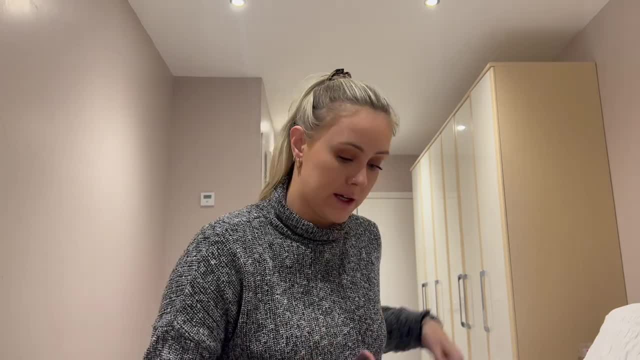 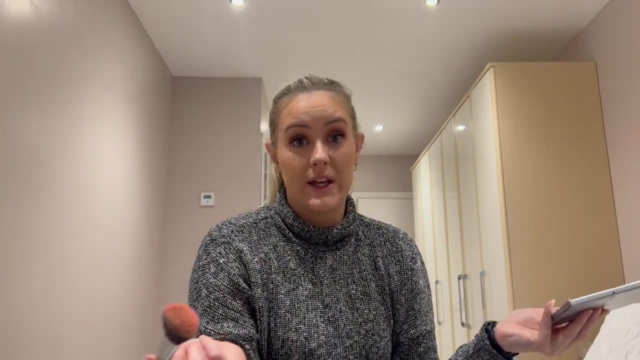 getting up to. It won't be very much lab stuff, just to give you a warning. but I will be kind of talking you through how my week is going and what I'm up to, just to give you a little insight into what a week is like as a research scientist. 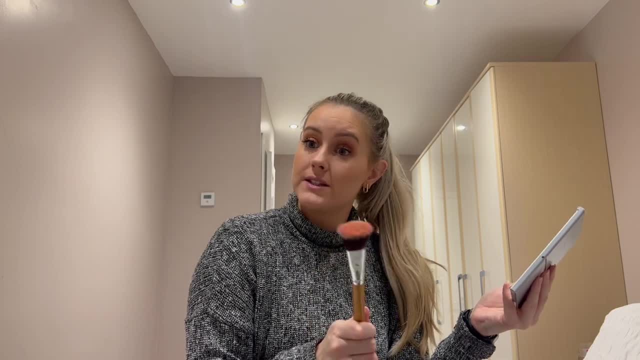 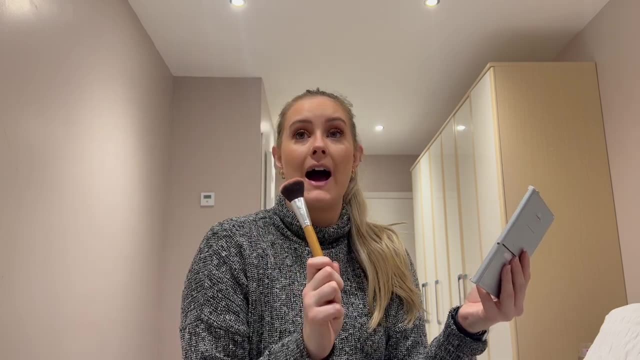 Enjoy. So the next time I'll speak to you will be in the office and I really need to get a move on, because it's five to eight and I want to be in the office by eight, which is not going to happen, but I need to do my hair still and, yeah, I'll see you at work. 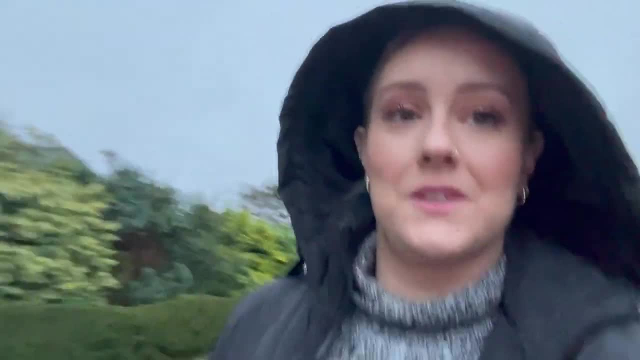 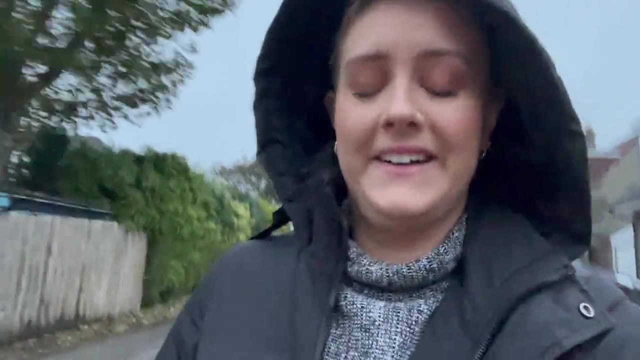 So just to give you an idea of what life is like in Scotland at the moment, it's eight o'clock and this is how dark it is, and it's cold and it's rainy. This is the beginning of the short days which I don't really love, to be honest. 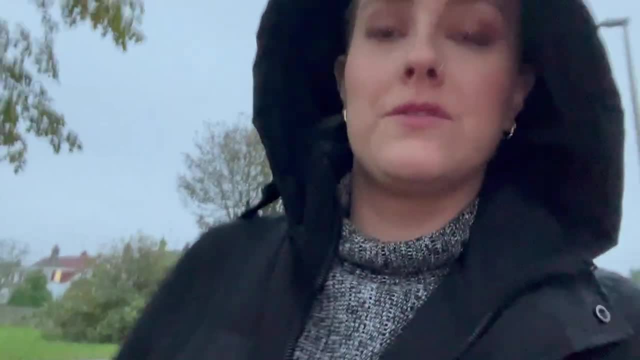 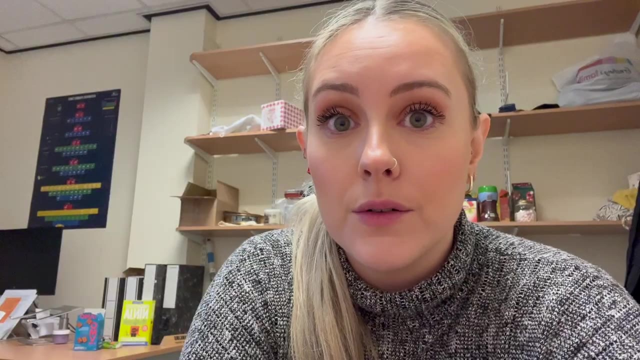 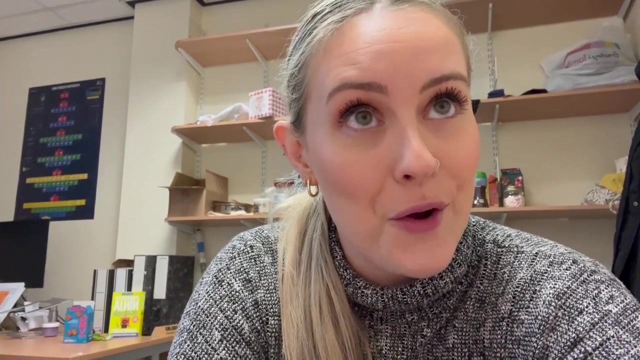 It's dark for a lot, a lot, a lot of the day, which can really take its toll. you know I am walking to work. I will speak to you when I'm at work. Hello, my friends, it is 10.44 and I am in the office. So this morning got off to an interesting start, so I actually 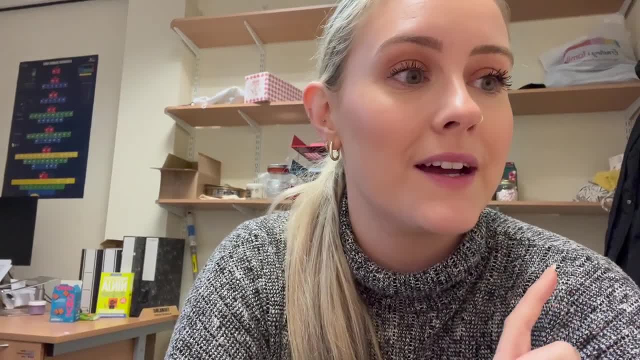 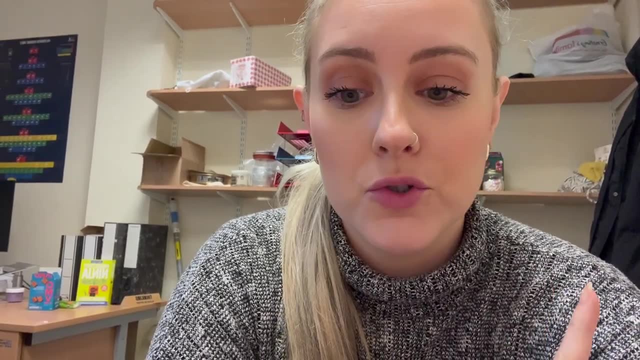 dropped my ID badge on the way to work and then had to retrace my steps to try and find it, and it was quite dark, as I showed you this morning, and I couldn't find it. I went back to my house, found said ID badge, couldn't find it, and then it turns out that a dog walker had actually picked up. 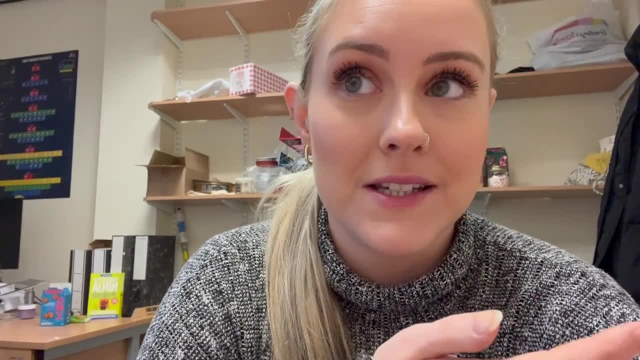 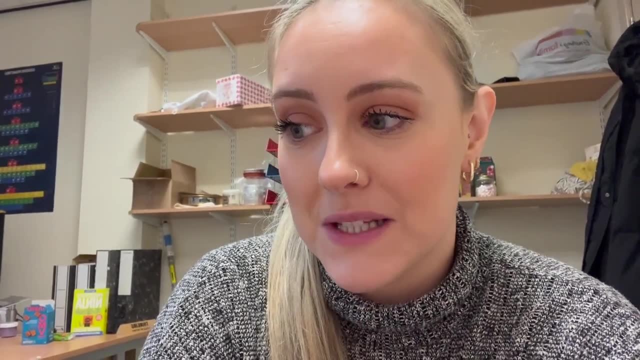 the badge and she saw me coming out of my house and asked me if I was Jessica because she had my badge. so I managed to find it, which was good. But anyway, since I've come in this morning, I have checked the instrument and it's still running. I had an email from my colleague asking if I can. 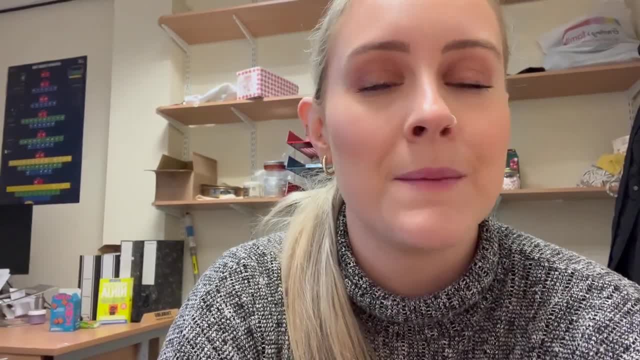 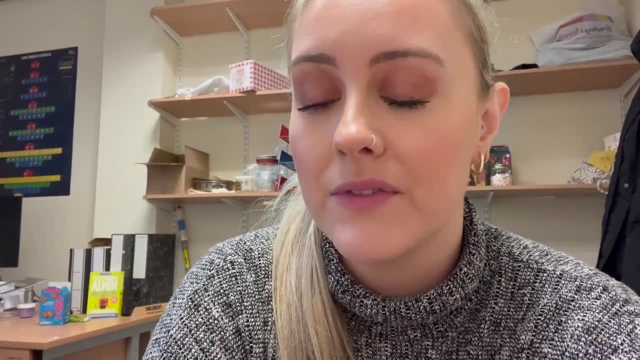 rerun some of her samples, because she's also going through data and there's one set of samples that doesn't look great. but I have to wait until this afternoon to do that because my sample is still running and it will be finished later on. But I have been sifting through my email since. 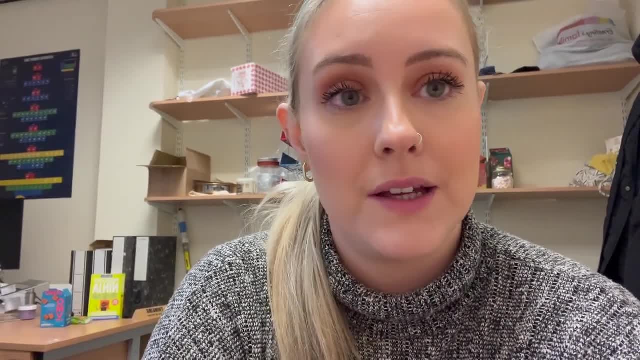 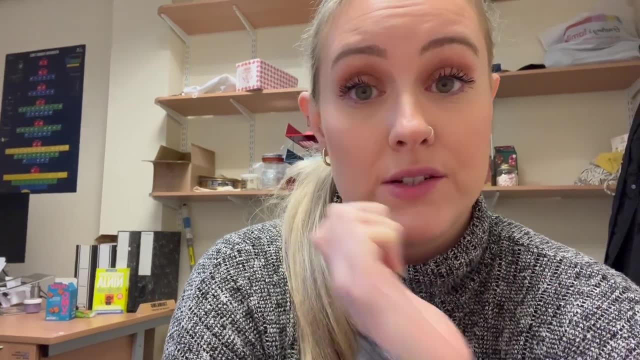 I've been off for a few days and I've actually been sorting out my application for my first grant that I am applying for, which is very exciting. I am basically applying for a small research grant to enable me to expand some of the current methods that we're developing into other 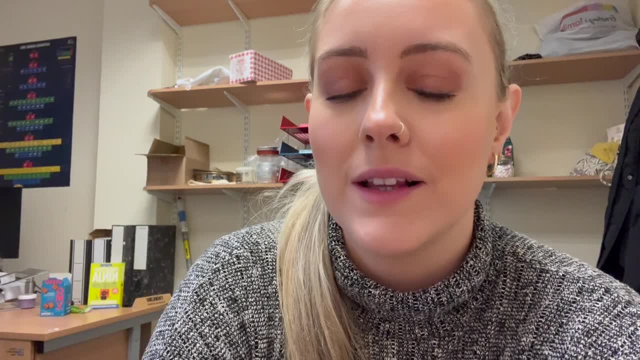 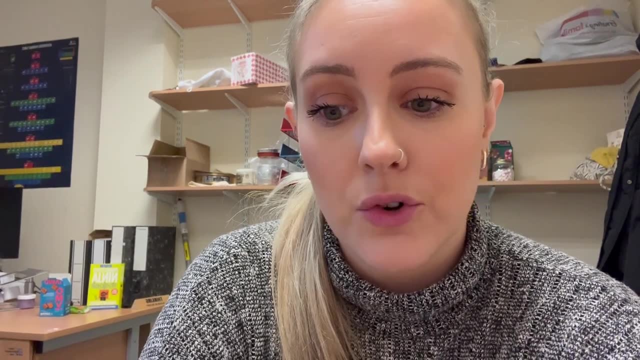 matrices, and it's quite exciting. I've been working on it for a while and the deadline is tomorrow and everything has kind of come at once, like I told you. So I'm trying to tie all of that up and I'll get it submitted later on today, But for now I am going to work. 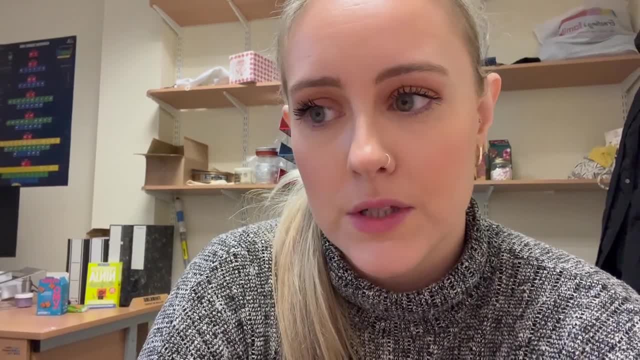 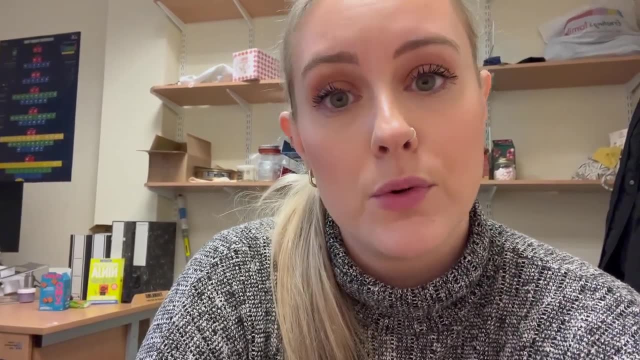 on processing some of the data that I exported. that was running, that was getting. what am I trying to say from the samples that were running over the weekend and yesterday? So I'm going to process those samples using the software for an hour and then I have a meeting at half past 12. 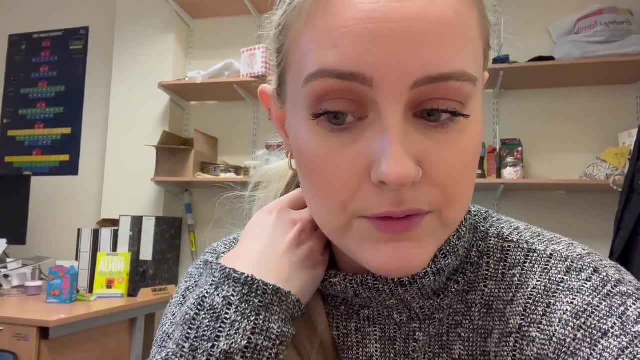 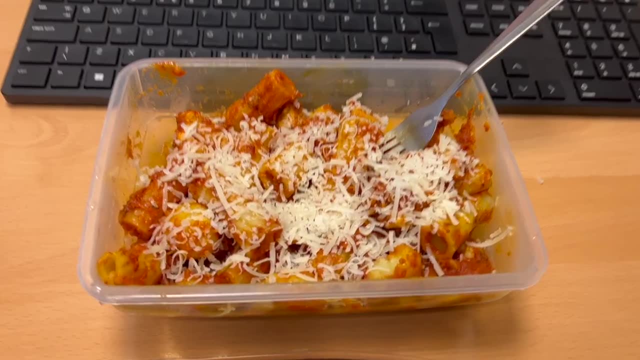 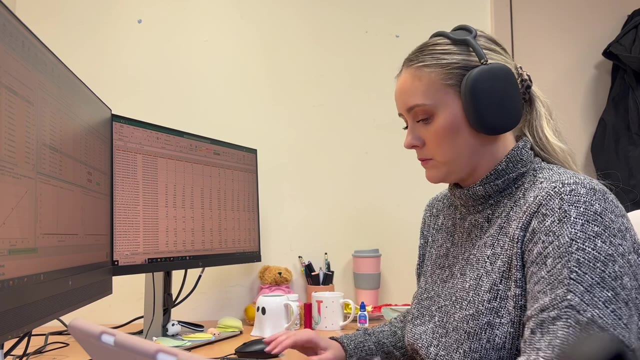 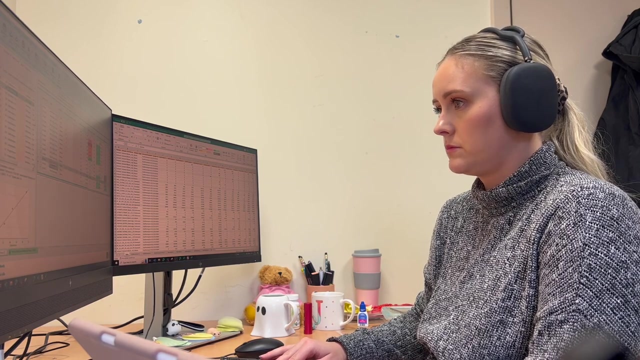 so I'm actually going to have an early lunch at 12.. So I'm going to prepare for that meeting for half an hour before I have my lunch and have my meeting and then back to processing data again in the afternoon. PLEASE LIKE THIS VIDEO AND SUBSCRIBE TO MY CHANNEL FOR MORE. 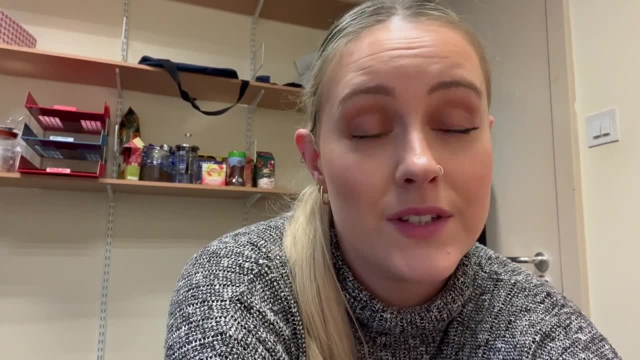 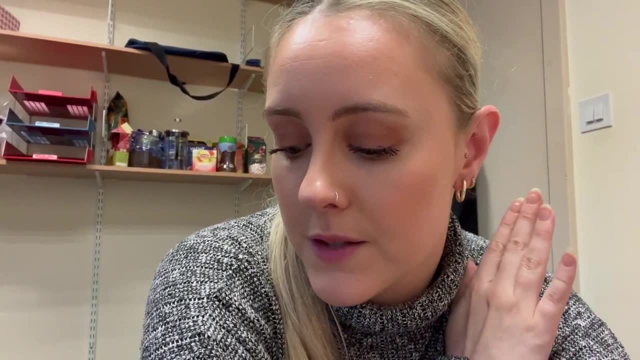 Hello, I am just checking in with you very quickly. I also need to give myself a little break from doing this data because my head is getting a bit sore. I do actually have blue light glasses, but I've been wearing my headphones and my headphones and glasses they push it. 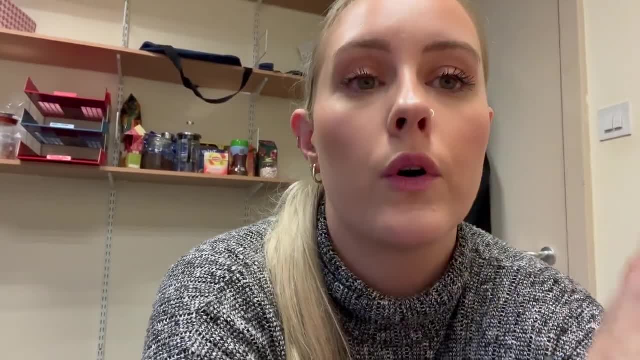 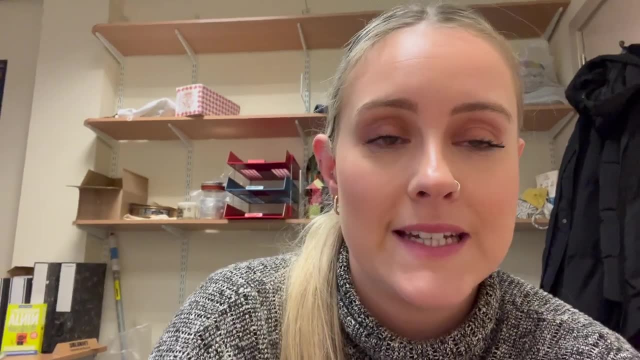 in my ears too much. i have changed my screens to be a more like warm color, so there's less blue light coming through. i'm watching a youtube video whilst doing my data. well, i'm like listening to it. i'm not watching it, of course. and yeah, i had a meeting. i haven't had lunch break actually to date. 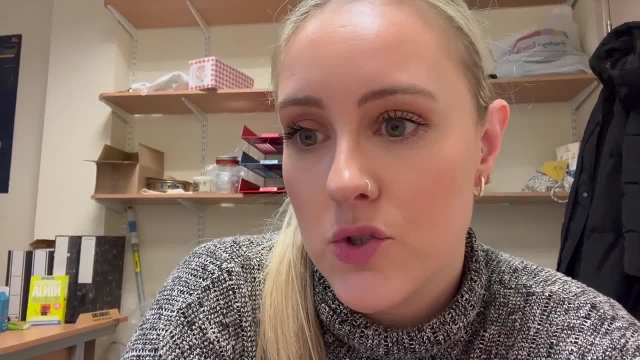 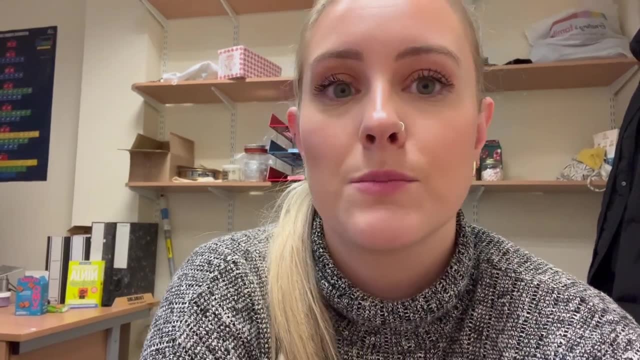 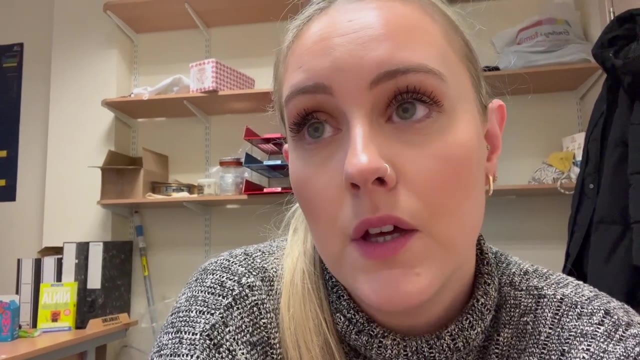 i usually would, but my meeting was at half past 12, so i ate my lunch while doing work from 12 until 12: 30 because my software was not responding on many, many occasions. so, yeah, that it means that i got quite behind with my data because the software wasn't working. so i am not quite on. 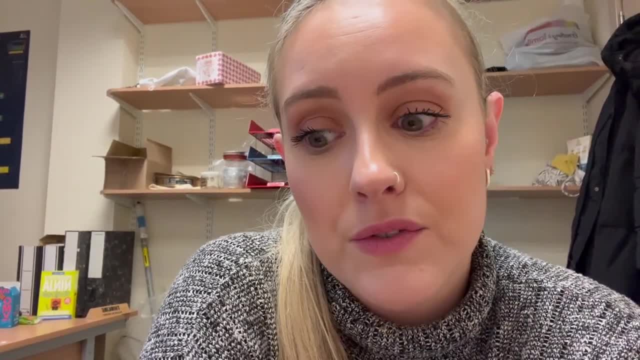 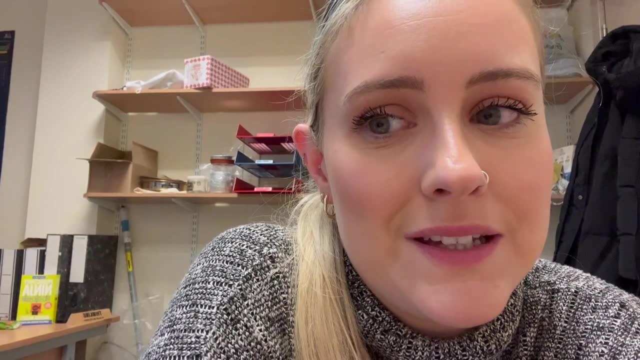 track for where i would like to be today, but i guess it's one of those days. the meeting was productive and i'm debating going for coffee time at three o'clock, but since i'll probably leave at four, i don't think i will go for coffee time because i also need to go to the instrument. 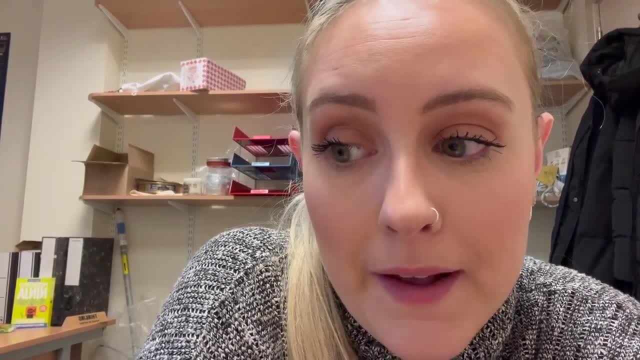 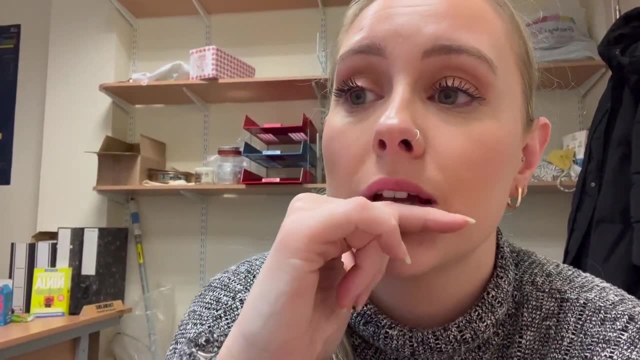 still and set it up for the analysis for my colleague um, which will take me a little while, probably take me from like three until four, to be honest. oh, i'm so annoyed that i'm not up to where i would like to be with the data today, but it is what it is, i guess. 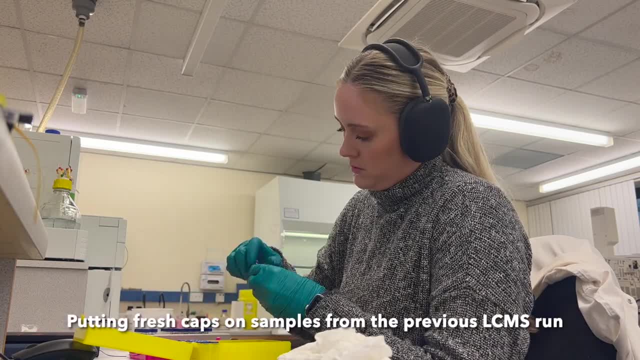 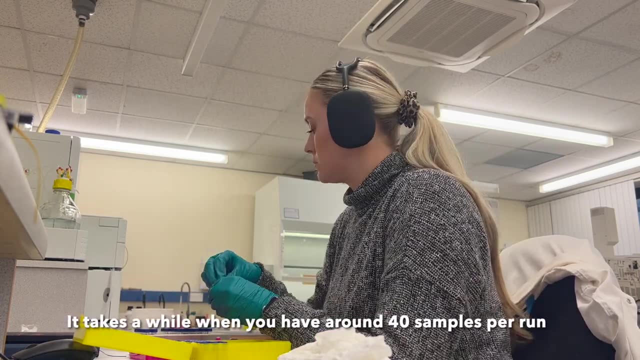 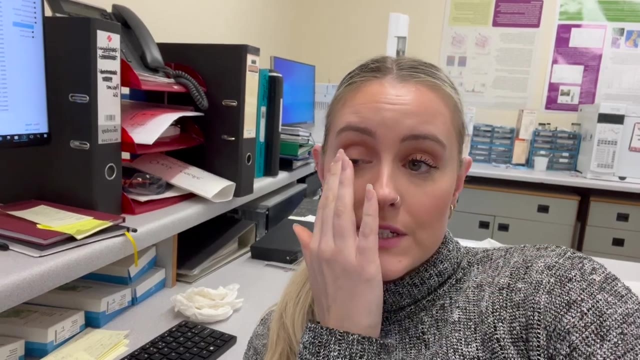 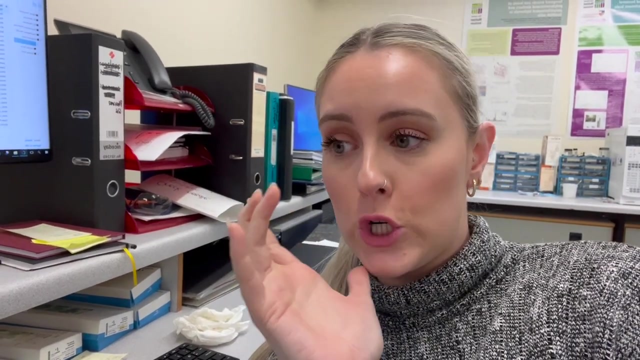 it is quarter to four. my friends, i have not finished my data. i have been swapping over the samples. i'm currently just well. i changed over the mobile phases. i've primed and purged. i'm running some of the new mobile phase through the column now. i'm then going to start the run. 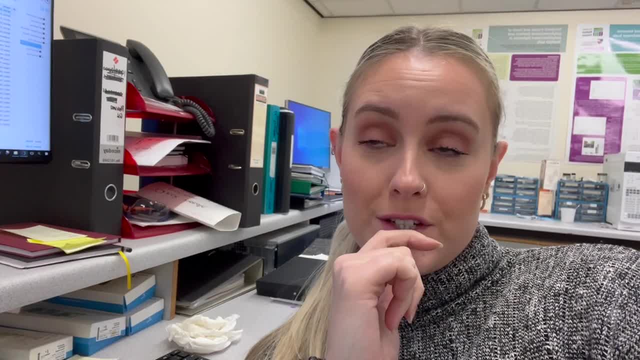 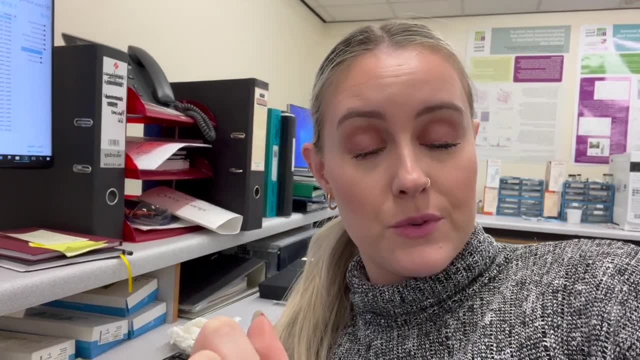 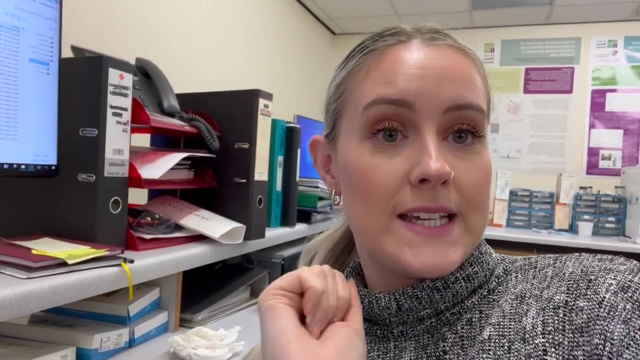 and and and And. then I think I I'm not going to finish at four o'clock, But I think I'm gonna go home because I'm quite hungry and I want to eat something, And I think I'm gonna submit my grant application from home And I'm also going to finish a little bit more data processing. so I can call it a day quite happily. 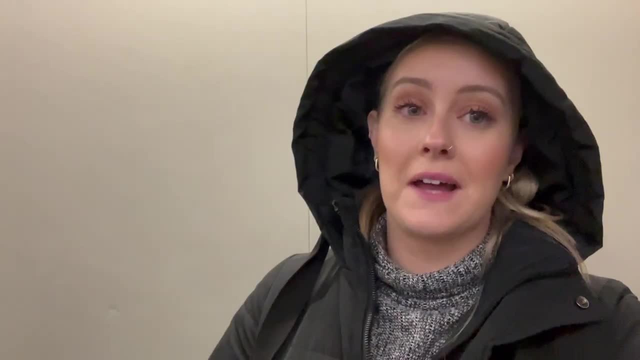 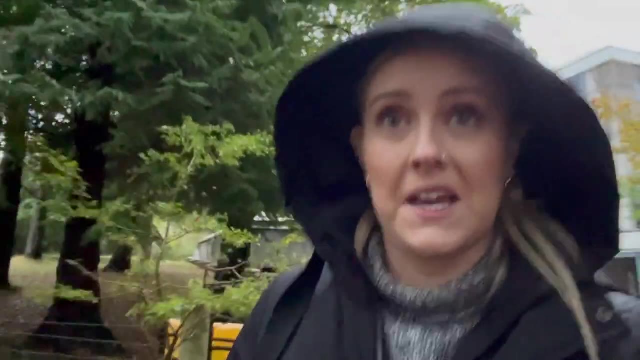 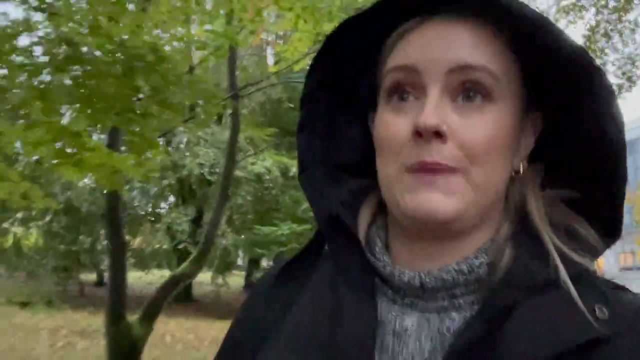 Guys, it is half past five, which is an hour and a half later than I wanted to stay today, But the instruments started playing up. Sorry that it's so dark, but it's half past five and it's a miserable day. But yeah, basically the instrument was leaking and I couldn't make it un-leak and it took me ages to fix it. 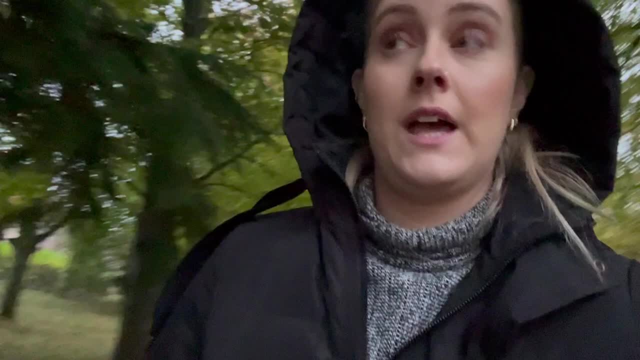 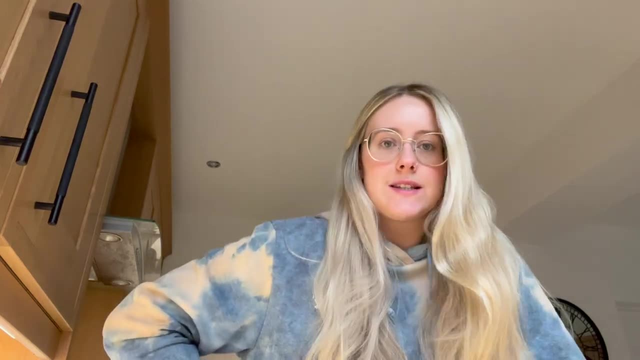 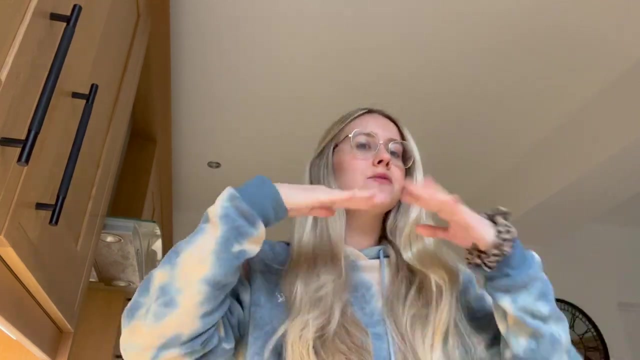 But I think I managed to fix it. now I put the samples to run. I'm going home. I will speak to you tomorrow. Hello, my YouTube friends, It is Thursday today, So it is the next day. Please excuse how I look. I have had a shower this morning after exercising. I washed my hair. I have moisturized. 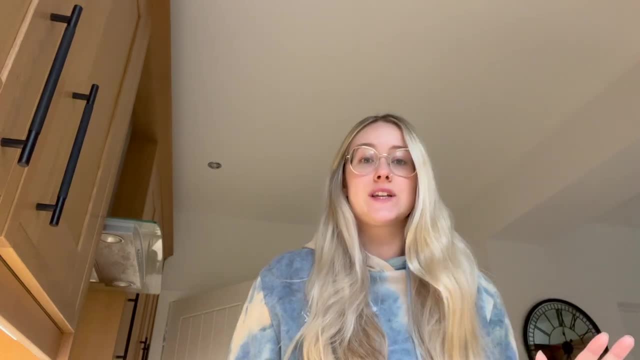 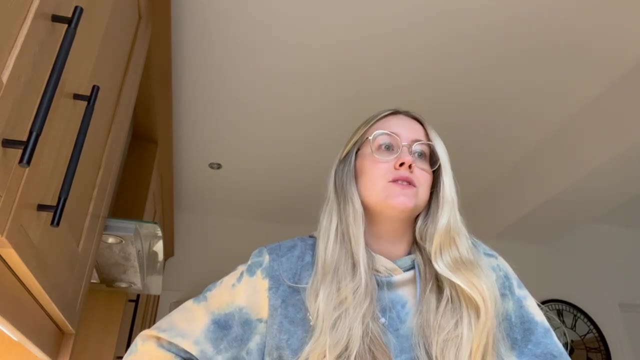 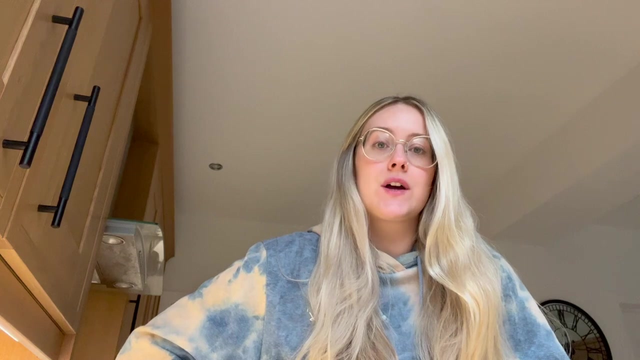 We are giving my face a bit of a break from makeup and contact lenses, So you're getting natural me today. As you can see, I am working from home today. I still have a lot of data to get through. just to put things into perspective: It is now half past twelve and I've been working since eight o'clock and I have only finished. 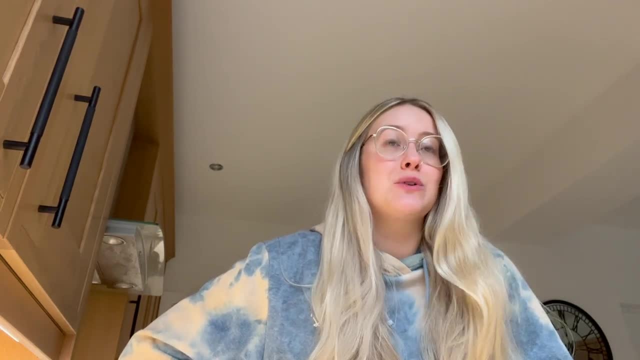 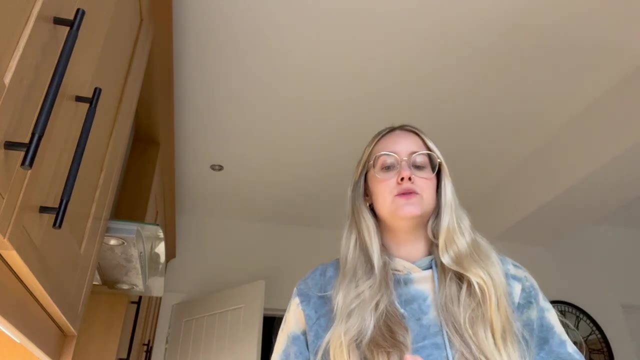 analyzing one sequence and doing all of the spreadsheets and all of the macros and Everything that has taken me four hours. I still have two more sequences to do. I still have two more sequences to do. I still have two more sequences to do. That's a lie. I technically still have four to do, because two of the earlier ones. 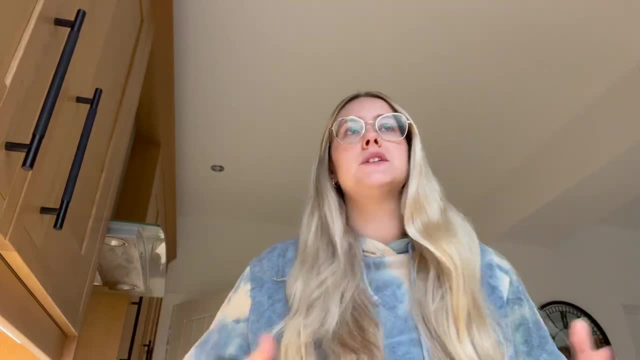 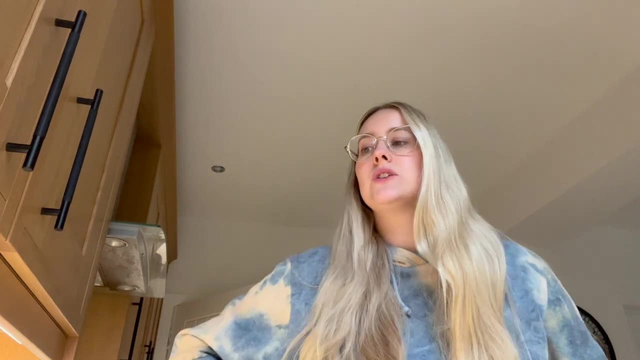 I need to reprocess and then recopy over all of the data and everything. so Technically I have four still to do. One data set- Oh no, I should have the data for that. The plan for today is. sorry, I'm a bit scattered. the plan for today is to try and get one more. 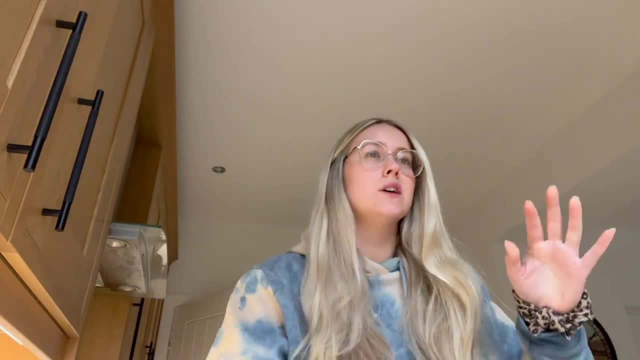 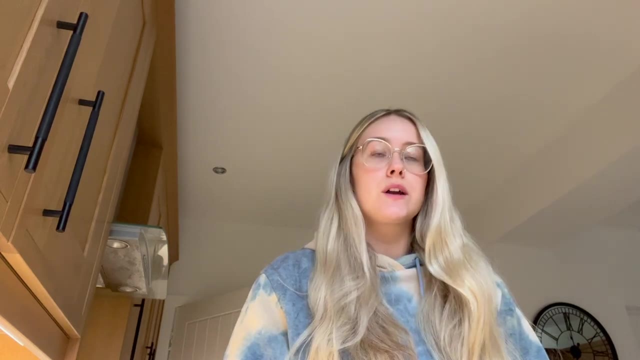 Finished and then potentially set up with a sheet with all of the information and stuff ready to do another one tomorrow. So half of the battle will be done will be done. I'm quite enjoying working from home. It is a dull, rainy, horrible day out there. 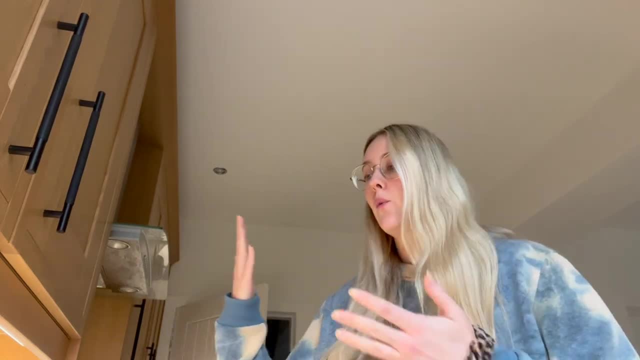 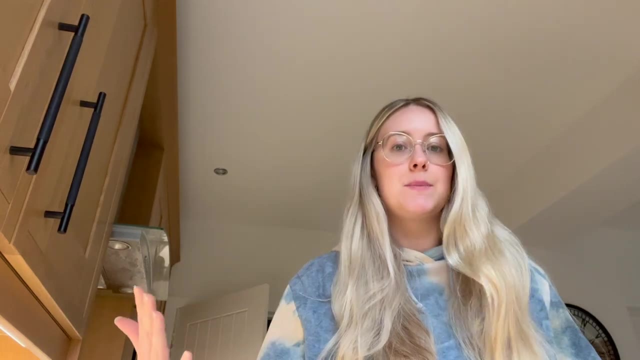 and I'm just working on data, so I might as well be, you know, watching a YouTube video doing my data on the other screen, getting multiple cups of tea, multiple snacks and happy days. Speaking of tea, I am currently making myself a cup of tea. I went on a bit of a shopping spree while Pete was. 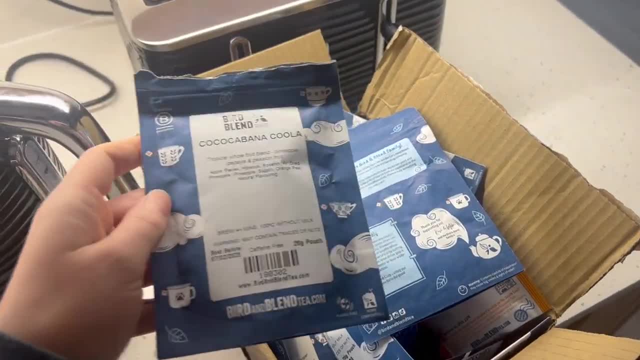 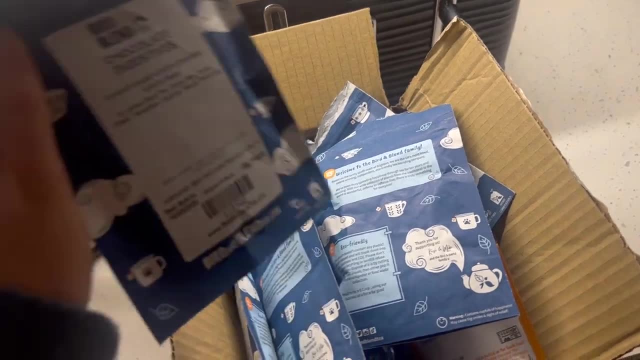 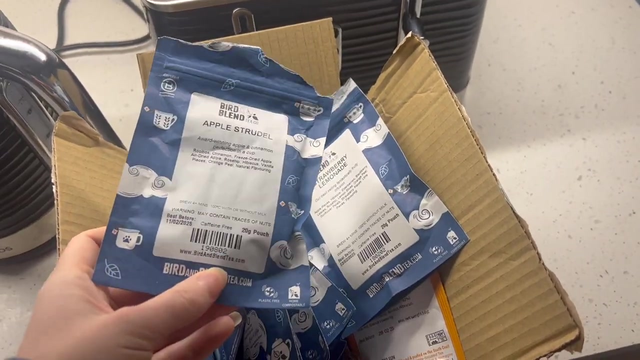 away and I was bored and I bought lots of like taster sizes of these Burden Blend teas. This is not sponsored. I just wanted to try a bunch of teas and they are supposed to give you 10 servings but I haven't actually managed to get 10 servings out of most of them, but I have lots of yummy. 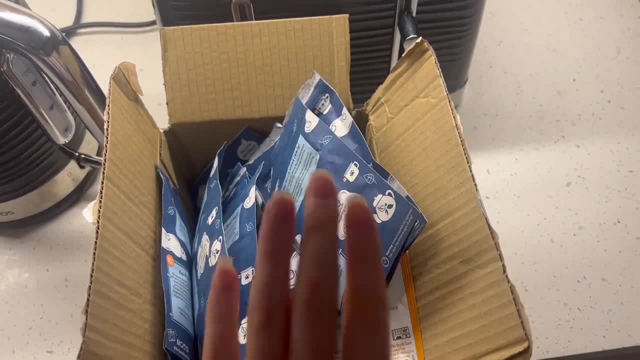 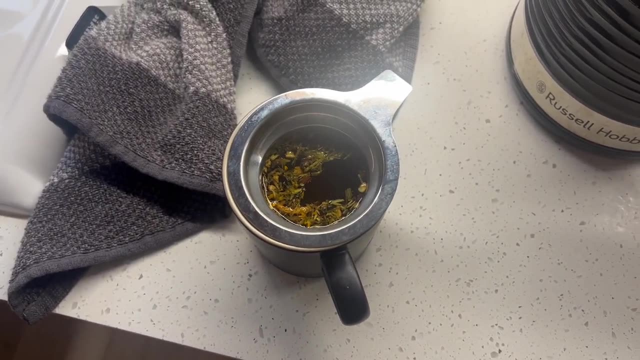 flavours, some caffeinated, some non-caffeinated, because I'm not always good with caffeine. Caffeine does make me a bit jittery and a bit anxious, but I'm just making a turmeric, turmeric, turmeric. why can't I say that? A turmeric tea just now? Where has it gone? I want to tell you what's in it. 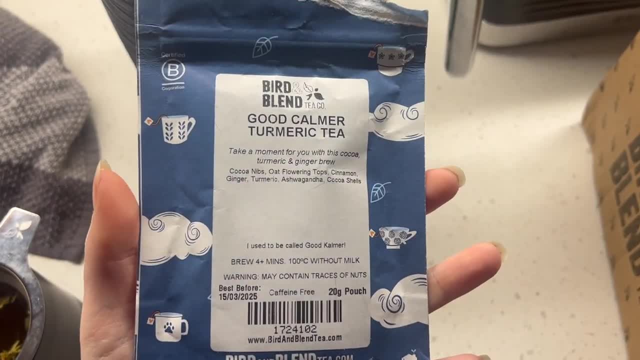 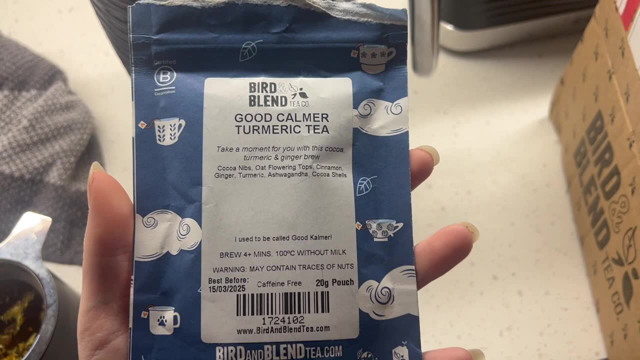 Here we go, The Good Calmer turmeric tea. So it's got cocoa nibs, oat, flowering tops, cinnamon, ginger, turmeric, ashwagandha and cocoa shells, and it's caffeine free and I'm going to drink that. 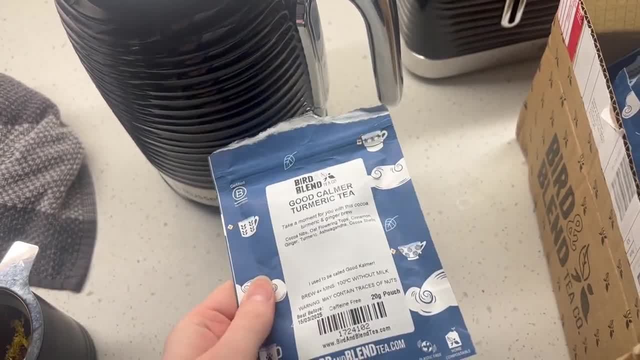 continue a bit of data analysis and then we will have some lunch. So just to put into context what I've been doing for the last four hours, I'm going to be drinking a cup of tea. I'm going to be drinking this tea. it's got mangoes and some mangoes in it, So I'm going to be drinking this tea. 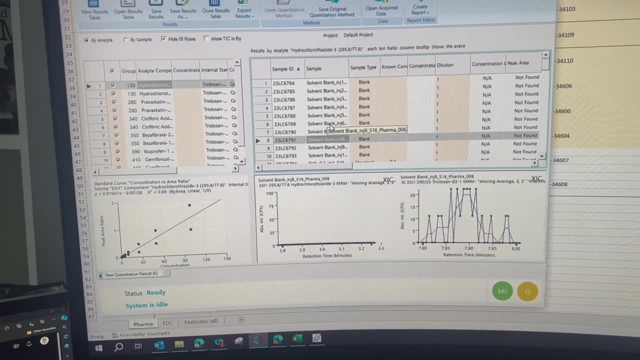 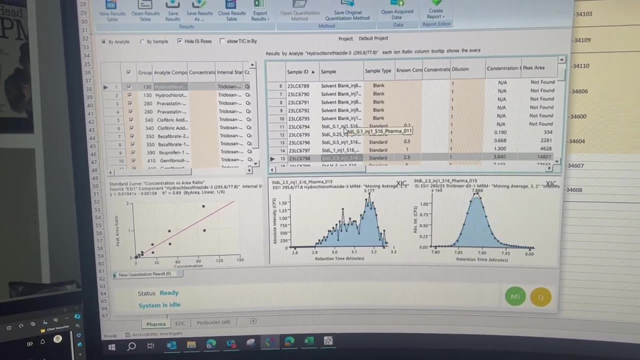 and I'm going to try to do the same thing. for the last four hours, I have been sitting here clicking through all of these samples to check for peaks and to reintegrate peaks if they don't look very good, And I've had to do this. So this is just one set of the samples for one compound. 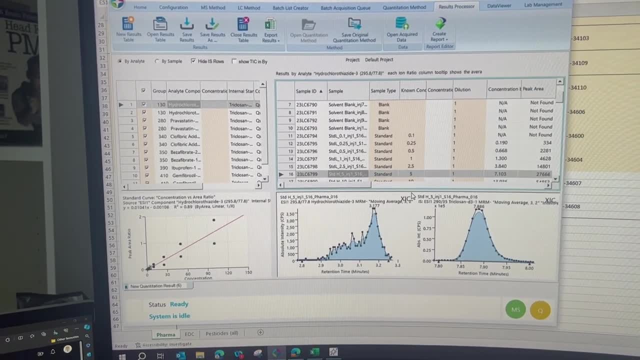 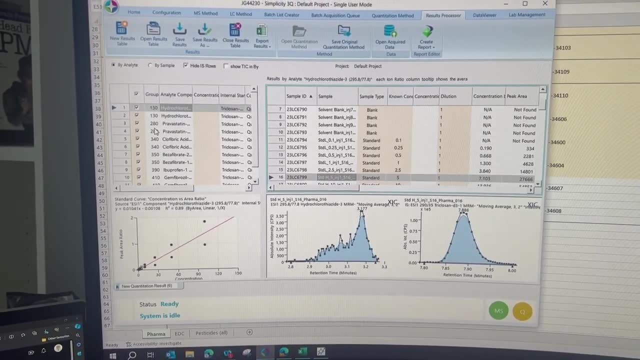 I've had to do this for 37 pharmaceuticals, So I have to check every single sample. There's about 80 samples in the dataset And then there are 37 pharmaceuticals. So if you do the maths to have a look at and then i have to copy and paste all the data into a spreadsheet, it's not. 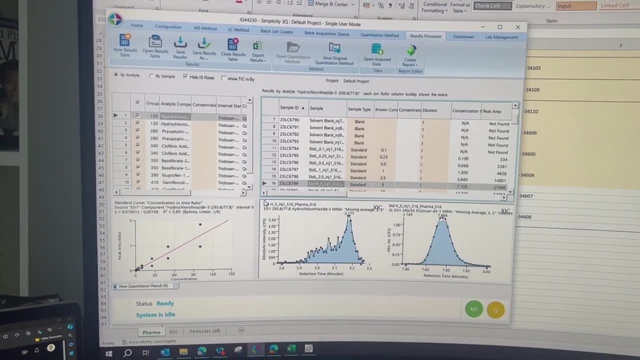 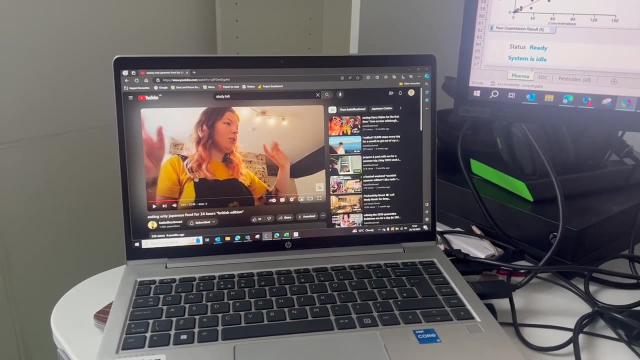 the spreadsheet and do macros and all sorts, and, yeah, that's why it takes a long time and that's why i have a youtube video on the go. i'm actually watching katie, who was my friend at school a very, very long time ago, and she has a youtube channel called katie likes bread and i'm catching up with 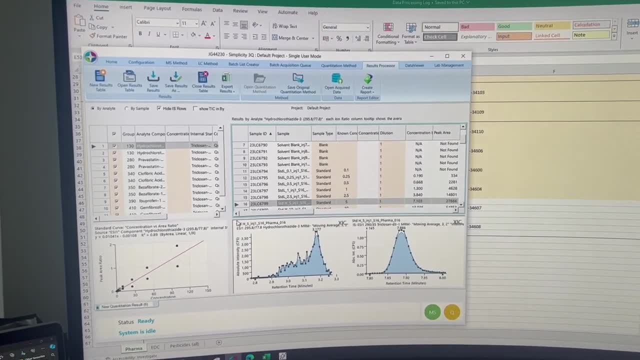 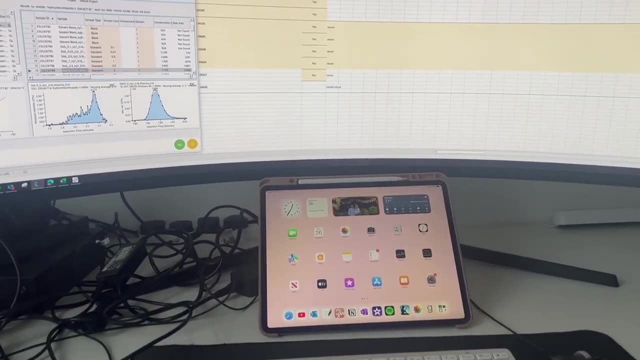 her videos and trying to not go insane doing this data. this is my computer setup, by the way. well, it's not technically mine, it's technically my boyfriend's, but now that we live together, what's mine is his. so i have a wireless keyboard mouse, ipad, because i'm going to start watching videos. 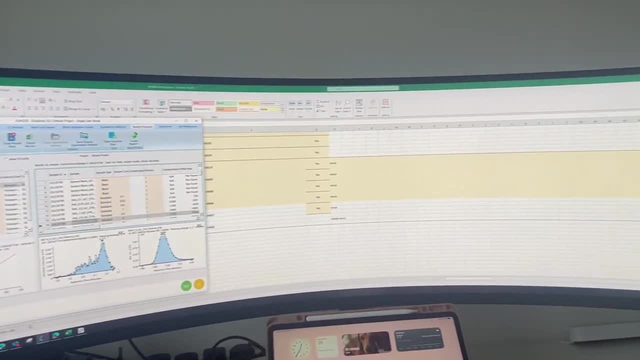 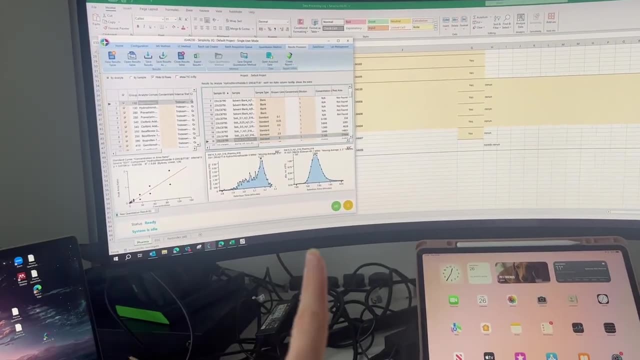 on here instead of here, because i'm going to use this screen and this absolutely massive monitor, which is very good when you're doing excel work, but i have to keep the software really small because if i make the software any bigger, it takes such a long time to go between the samples. 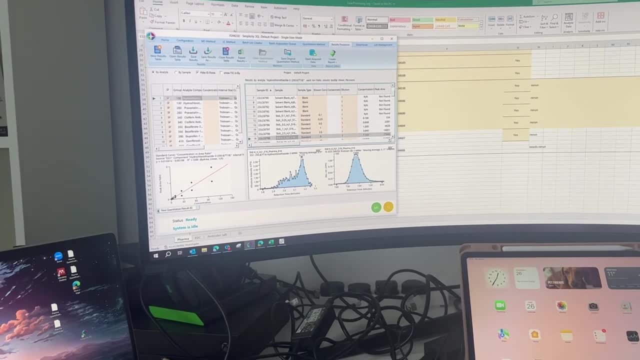 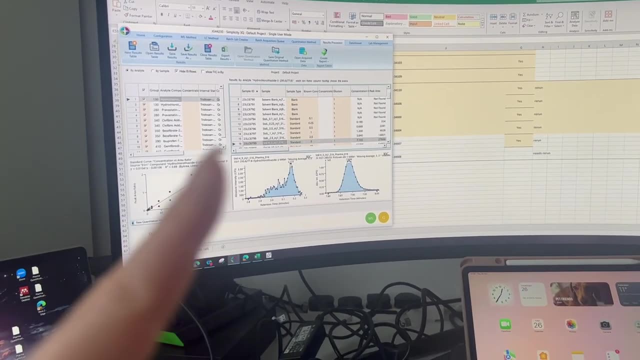 like for them to load. i don't know why that is, but it's highly frustrating and i need to use this tiny little window when i've got this massive screen, which doesn't make sense. but yeah, i can't be waiting five seconds in between each sample when i have a lot of samples. 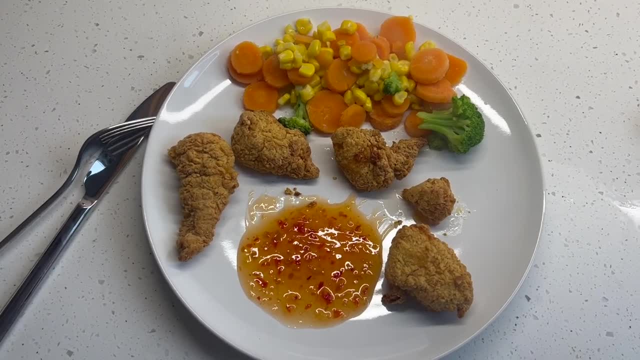 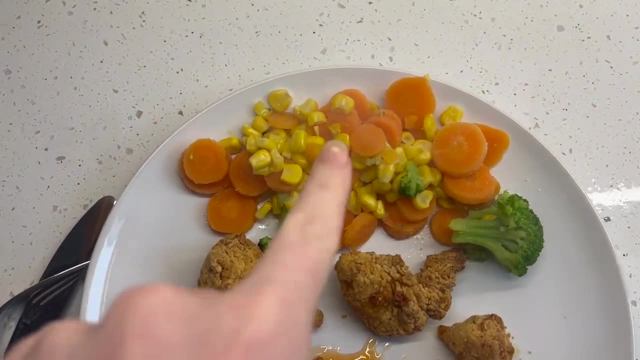 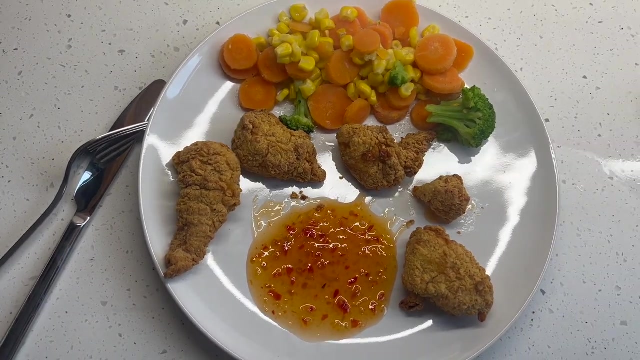 that i need to look at. okay, so it's lunchtime, it's 10 to 2 and i'm having these little flaming hot chicken tenders from costco, some hot sweet chili sauce and some microwave in the bag of vegetables. this is the definition of a quick and easy, no cooking, no fuss lunch i'm going to eat. 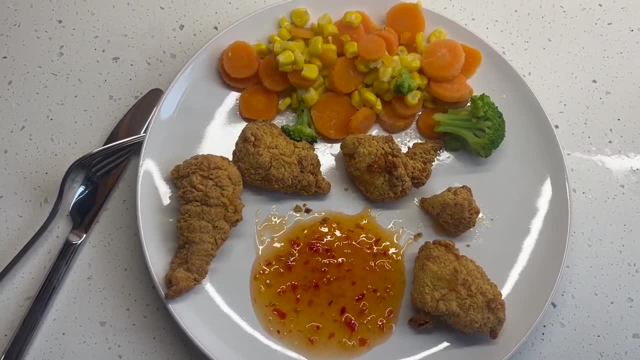 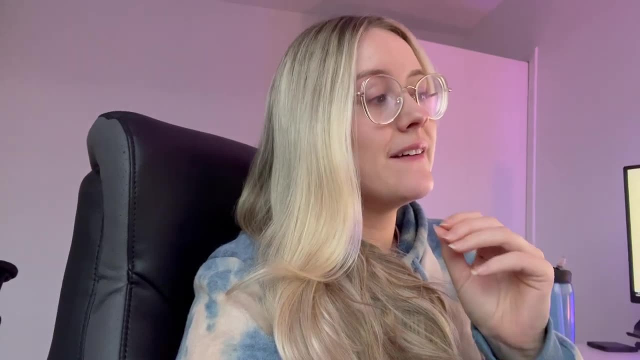 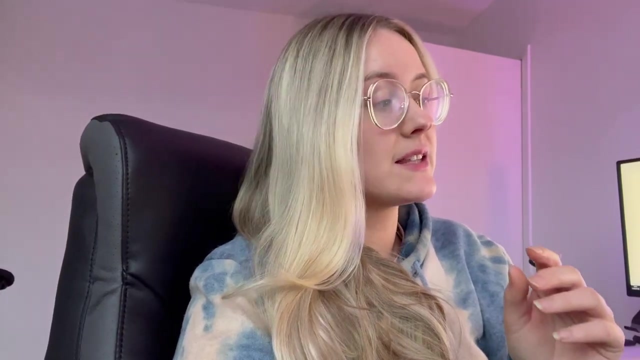 this and then we're going to get back to the computer again to do more data analysis. hello, i'm going to get my second sequence of data finished. i don't know what time i'm going to work till today, because i have recently been working quite a bit of overtime and i'm feeling. 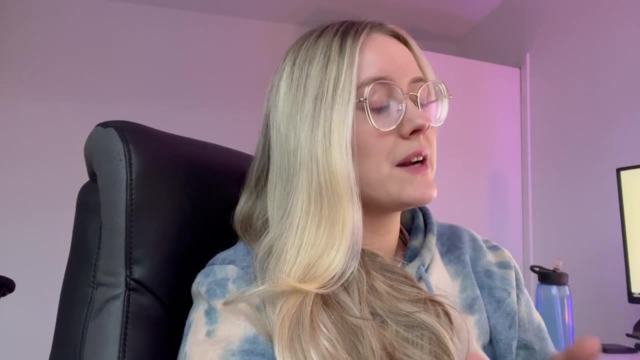 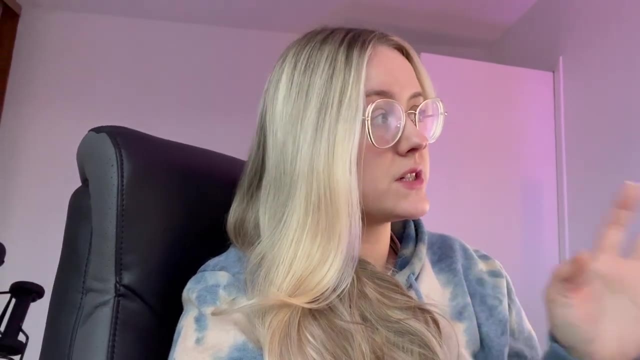 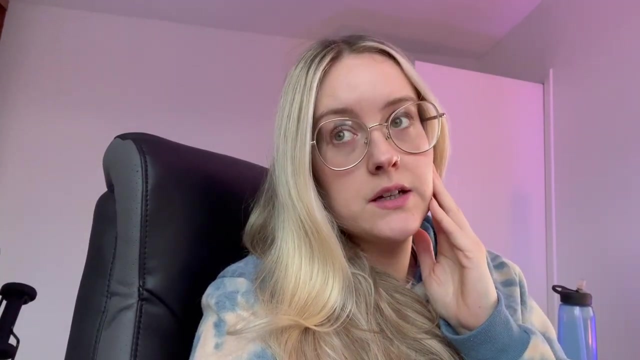 100 today, to be honest with you. so i might try and finish at four, so we'll see how much i can get done. i really want to get this second sequence analyzed and all the data copied across. i'm doing the spreadsheet stuff now with all the numbers and if i have some time until four then i can. 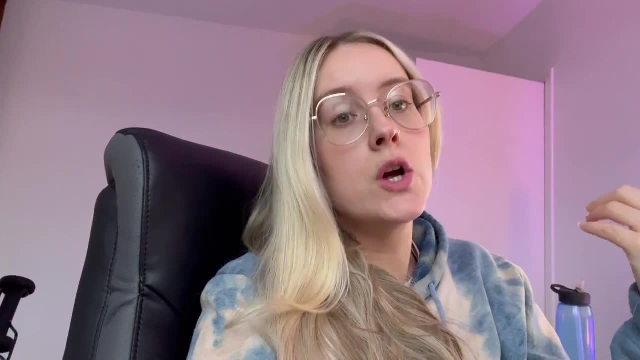 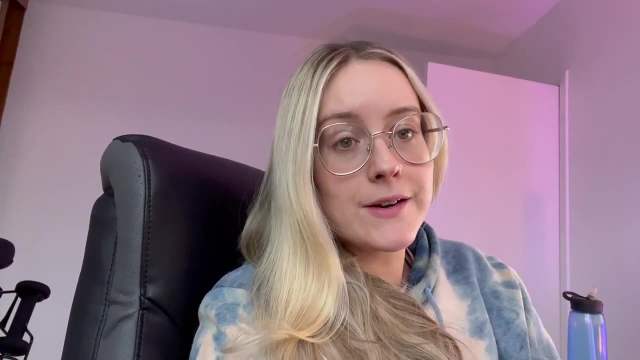 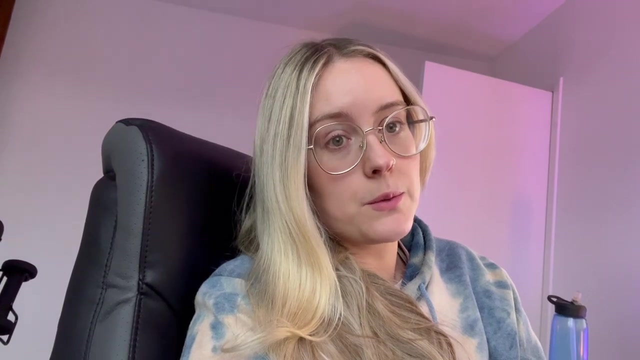 do some other bits to prepare for my day: data processing for tomorrow. i think i'm going to go into the office tomorrow just for a bit change of scenery, to keep me inspired and motivated. but yeah, i don't have a sore head yet, which is good, but i do feel like i need a little five minute break from the screen. 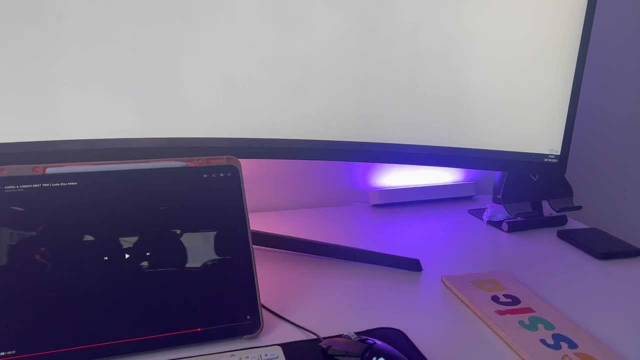 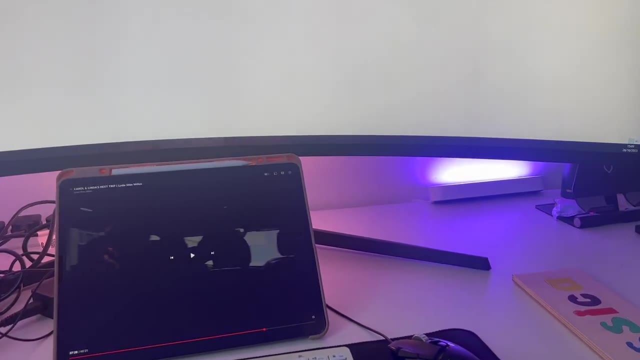 so i know i already showed you the setup, but it's beginning to get dark outside. it's three o'clock so i've put lights on and look at the colors of the lights. i've got this like galaxy theme on the philips hue lights. these are my boyfriend's philip hughes as. 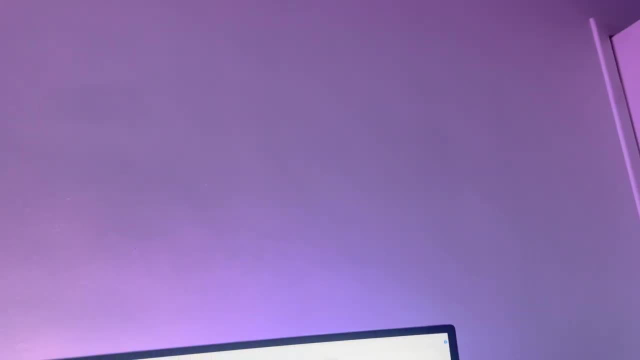 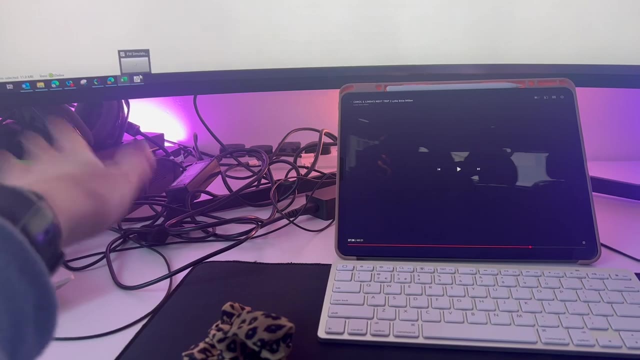 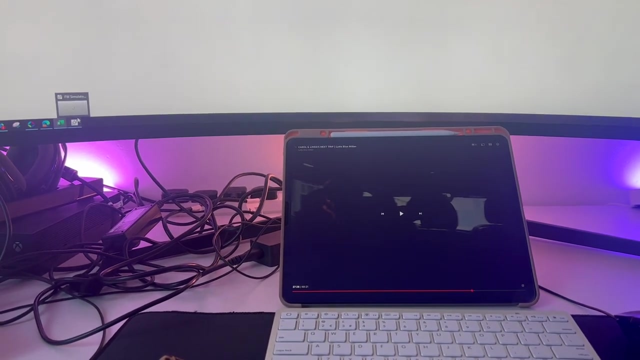 well, and it just makes such a nice glow and gives a little bit of ambiance. ambiance, uh, for doing my data processing. this situation needs sorted, though all these cables is. they're kind of giving me anxiety. right, i am actually going to meditate for five minutes and then i am going to 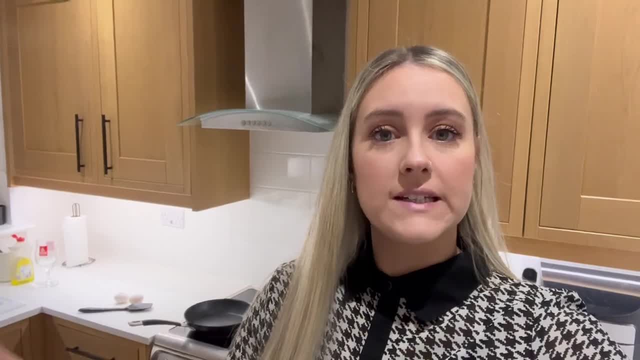 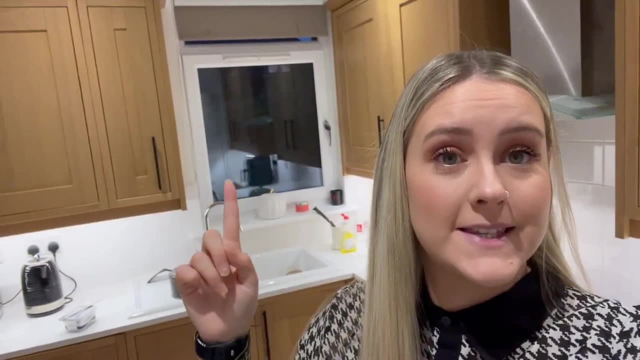 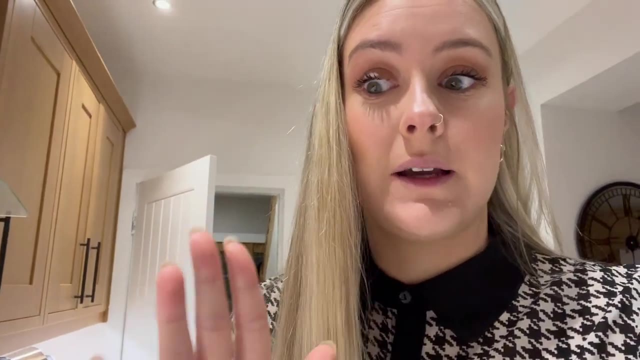 resume my data. hello my friends. happy friday. we're going into the office today. i'm about to cook some eggs and some toast. these spotlights are not great but, as you can see, it's pitch black outside and it's eight o'clock. i'm struggling with these very, very dark mornings. i'm not going. 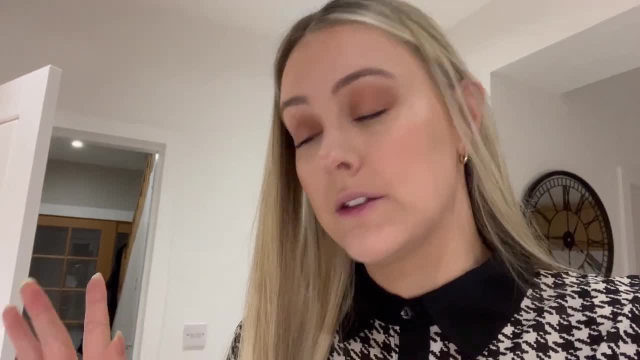 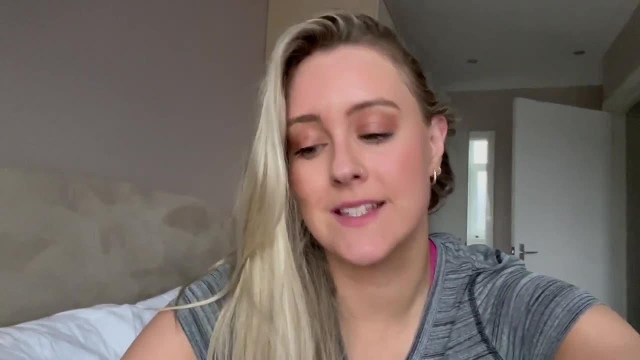 to lie to you, but let's make the eggs and hopefully we can get into the lab for quarter past eight. hello friends, i'm currently looking a little bit like a tomato because i have just exercised, because it is actually half past four and i forgot to update you guys during the day today because 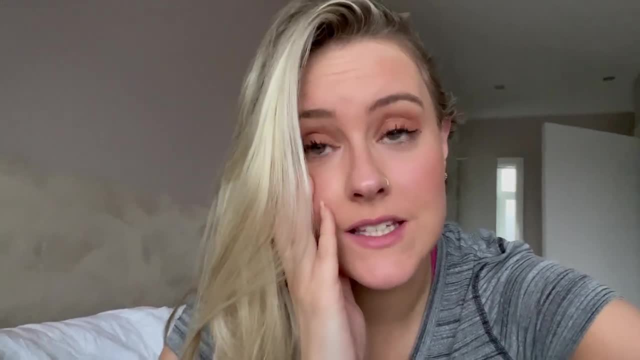 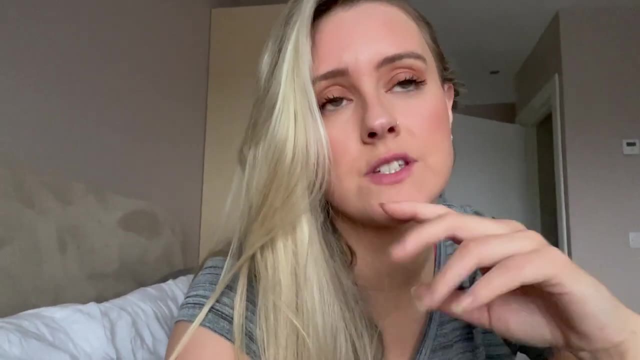 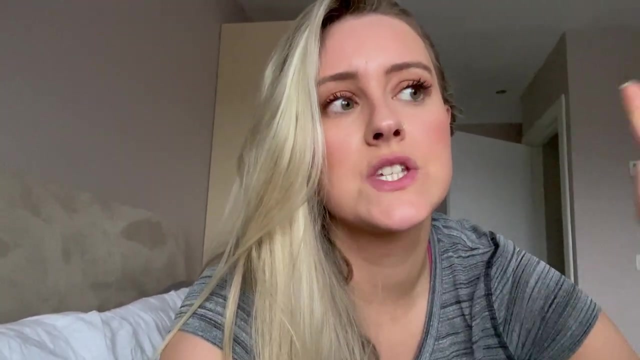 it's been actually quite busy and not just data orientated today. so to give you a little lowdown, i got to work at eight o'clock, just after eight, and i caught up on my emails and i noticed that my supervisor actually wanted to have a catch-up meeting in the afternoon, so i scheduled that into. 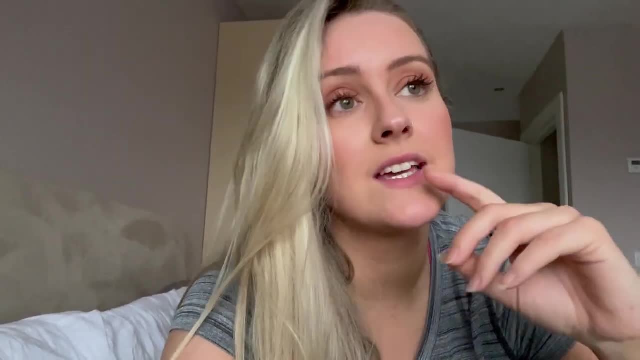 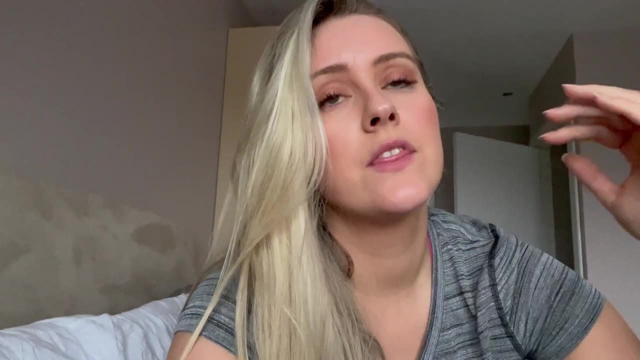 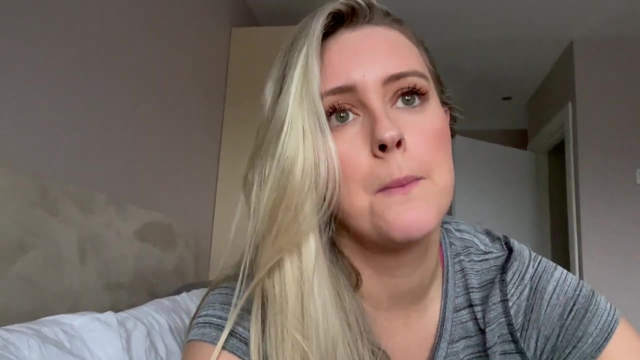 my plans for the day. then i started, uh, analyzing my data, managed to get through one of my sequences and then i had a meeting at 11 o'clock with perkin elmer, who is actually the company, the brand, of our lcms instrument, and basically because we have a service contract with them and because we are a 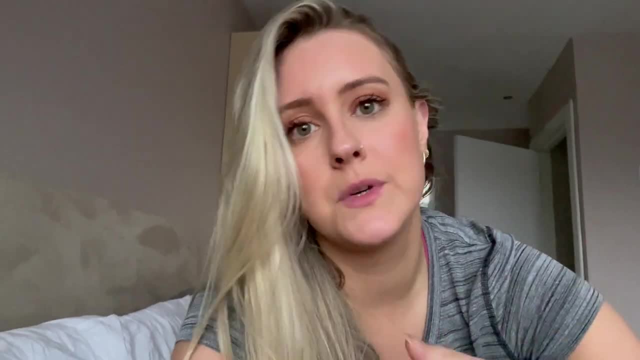 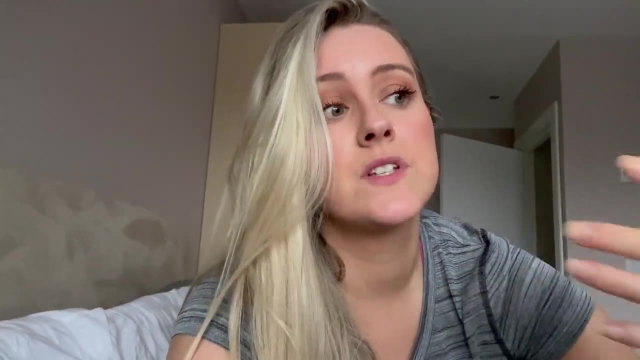 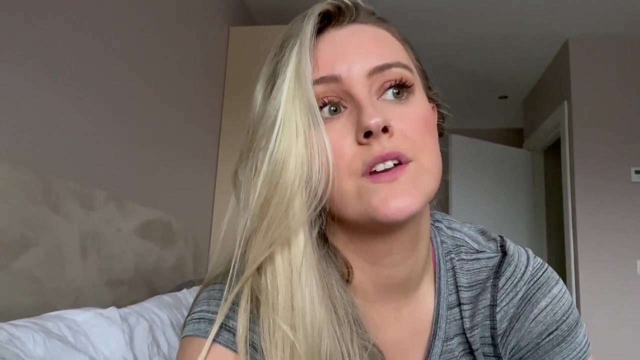 user of their instrument. we have a service contract with them and we have a service contract with they're very happy to help us out when we are developing new methods. so i can have meetings with their technical support team, who are constantly developing their own methods for new and emerging contaminants that they want to analyze. so i had a meeting with one of their 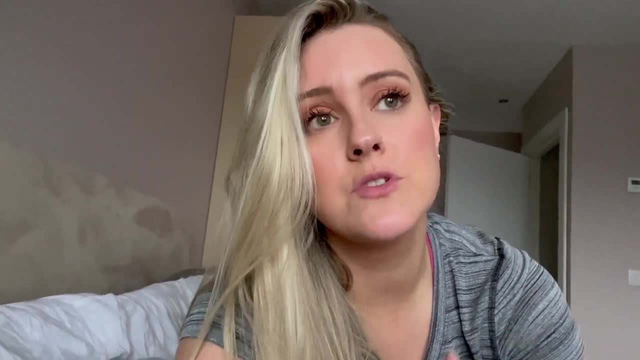 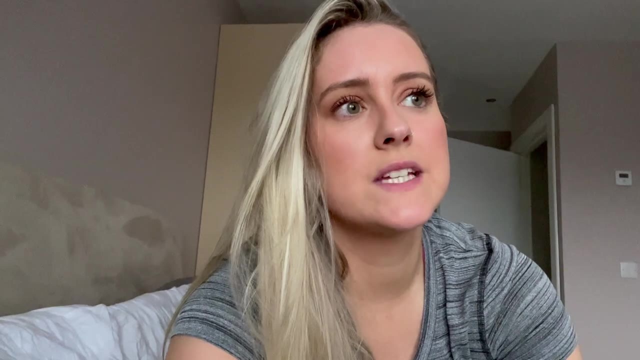 specialists and we were just having a chat about some of the analysis that i'm doing and some of the analysis that he's doing and how we can help each other out, so that was good. i was on in that meeting for about 45 minutes and then i did some more data analysis and then i had a meeting with 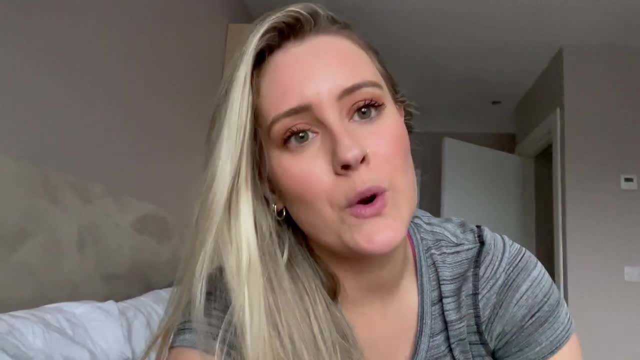 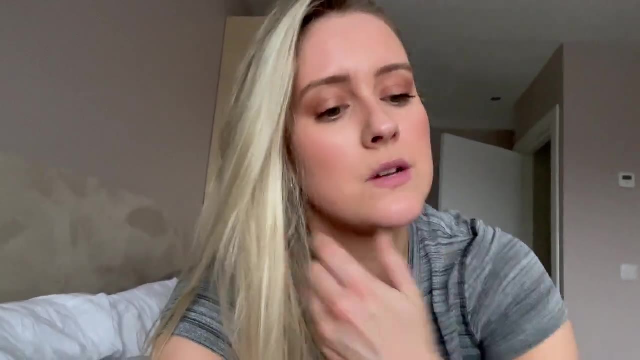 data. and then i came home for lunch and then i went back to work because i had my meeting with my supervisor and that was fine. he just told me that he is basically he's going on holiday, and i told him that i'll have the data for him and all of my graphs by wednesday next week. so did i say?